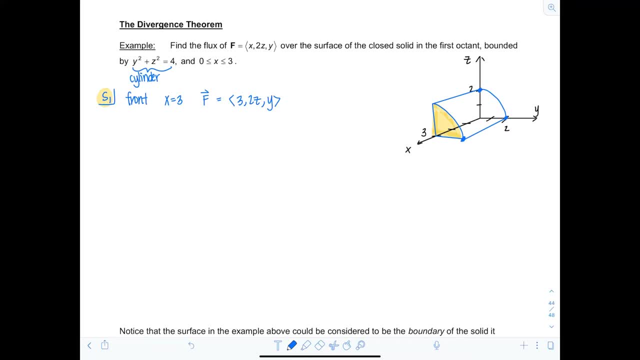 Would be 3,, 2Z and Y. And then I need my outward unit normal. So outward in this direction- just imagine it would be pointing in the positive X direction. components would be 1, 0, 0.. That means f dotted with n would just be 3.. Okay, so the flux on that. 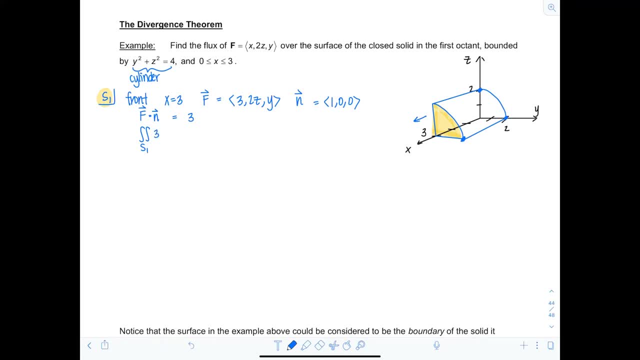 first surface would be surface integral over surface 1, 3 ds, which would just be double integral over d1, which would be in the yz plane of 3 da. So it's just 3 times the area of that region in the yz plane that the surface x equals 3 lives over. And if you can look here: 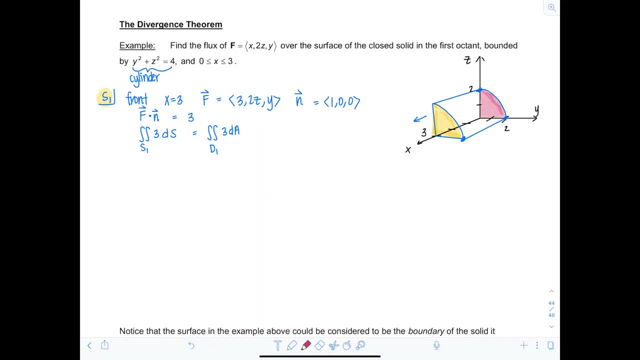 right, it's just a quarter of a circle. So I'm going to take 3 and then multiply by 1, fourth times the area of a circle with radius 2, which would be 4 pi. So the 4s cancel out and I get 3. 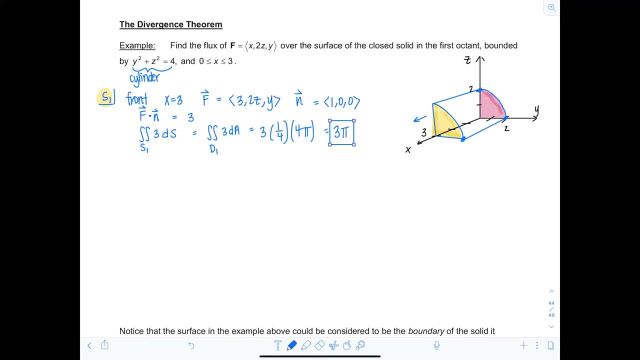 pi. All right, very good, So that's done. Surface 2, we'll say, is the back? Okay, and it's actually already highlighted in, so I'll just use that same color there. The back is determined by the plane. x equals 0.. 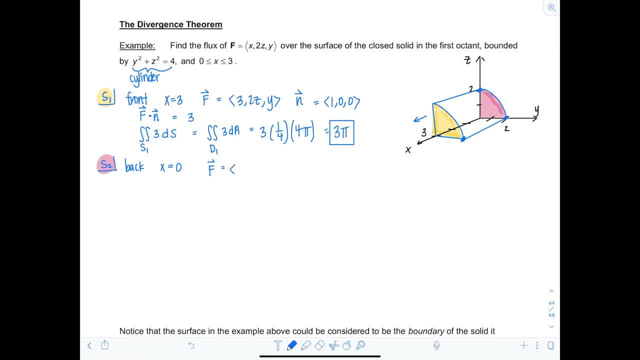 So my vector field on that plane is defined to be 0, right, substituting that in for x, 2z and y. And then, remember, our normal has to go outward, So the normal vector would point the negative x direction, so it would have components negative 1,, 0,, 0.. All right, so fn. 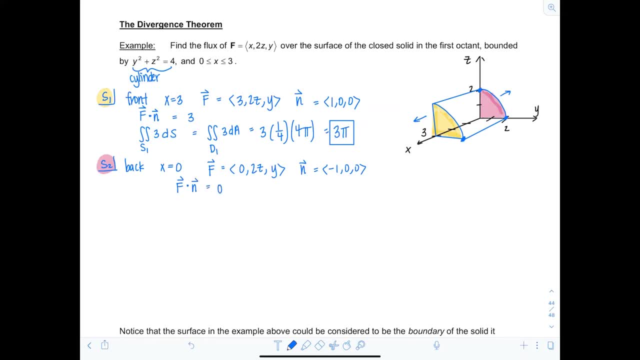 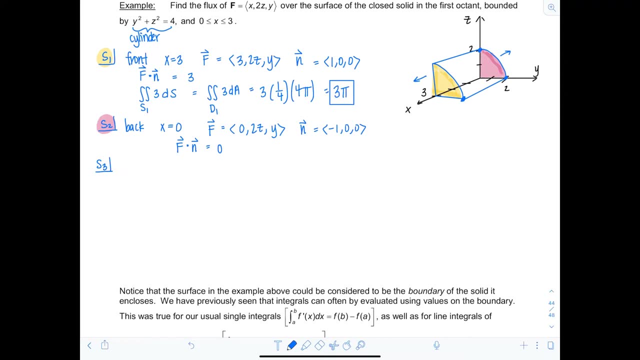 on the back is just 0. So the flux is going to be 0.. No need to do anything else. All right, what about surface 3?? I told you there were 5, right, So surface 3, I'm going to say it's this. 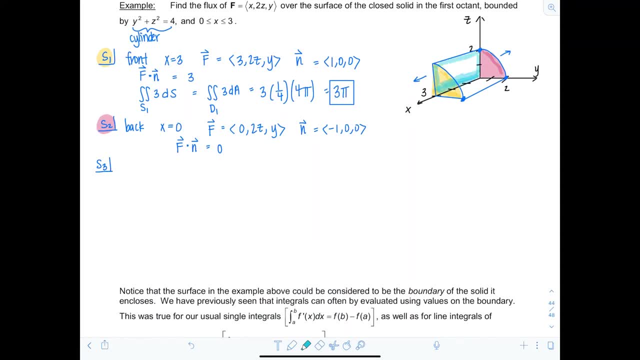 left side. here this rectangle. Okay, I'll color it in here, so everything's matchy-matchy, so you can find it. So the left surface is determined by the portion of the plane y equals 0. My vector field on that surface, substituting in 0 for y, would be x, 2z, 0.. Okay, what's the? 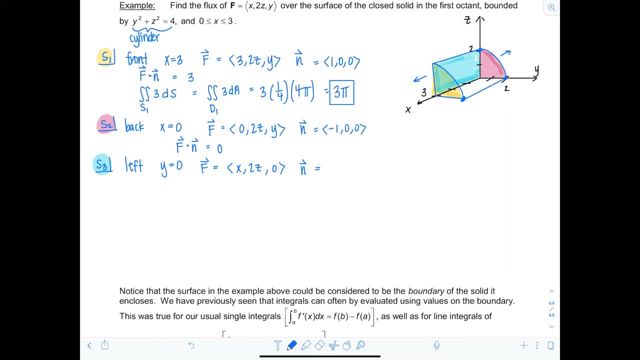 normal vector to that surface. Outward. outward, It's going to point in the negative y direction. yes, So the components would be 0, negative, 1, 0.. In that case, fn, we can compute. fn is going to. 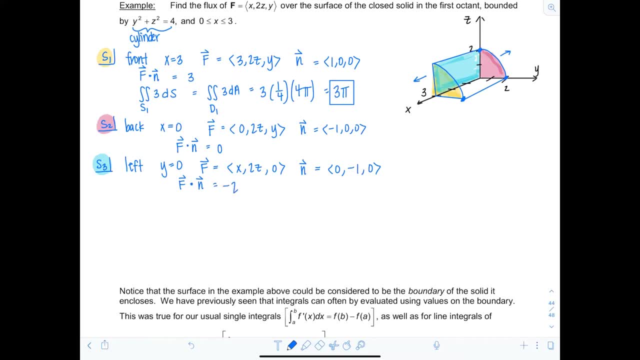 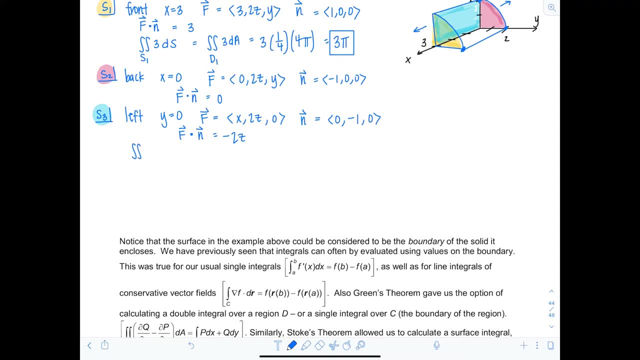 be 0 for the first component, then plus negative 2z plus 0.. Good, Okay, so this we have to actually evaluate now. So surface integral over surface 3 is going to be negative 2z ds, So it makes sense. 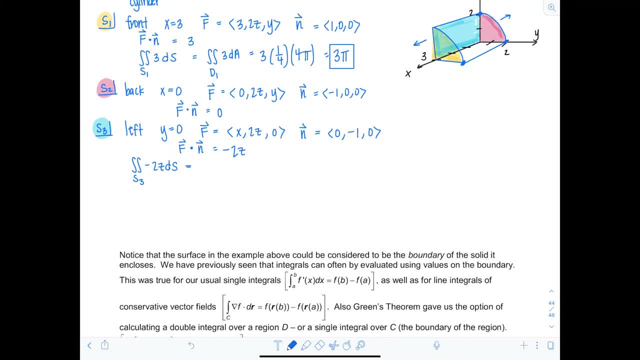 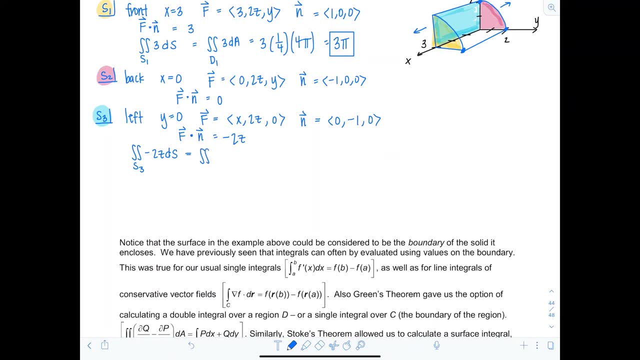 It makes sense. I'm going to integrate this surface over that rectangle in the xz plane. Can you see it? It's pretty straightforward. So we're going to have double integral over, I'll say, some region d3 in the xz plane of negative 2z da. 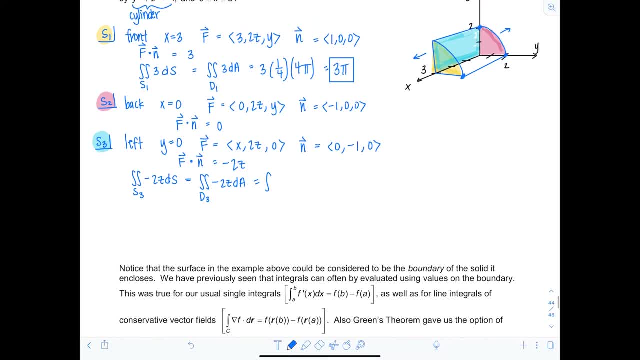 And then the limits. look here, it's just a rectangle. So limits for z are going to be from 0 to 2.. Limits for x would be from 0 to 3.. And then I have negative 2z ds. And then I have negative. 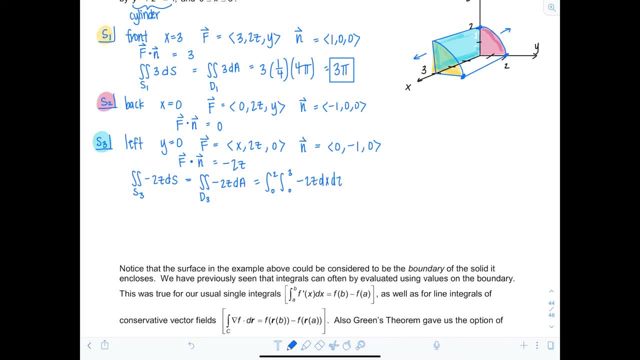 2z, dx, dz, And this gives us negative 12.. Okay, very good, We've got two more surfaces to go. We can do it. So surface 4,, surface 4,, I'll call it the floor. The floor is going to be. 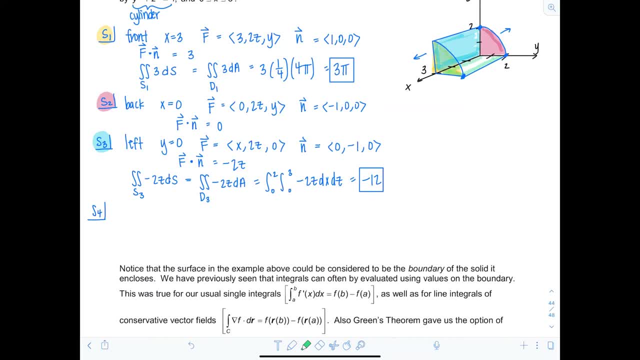 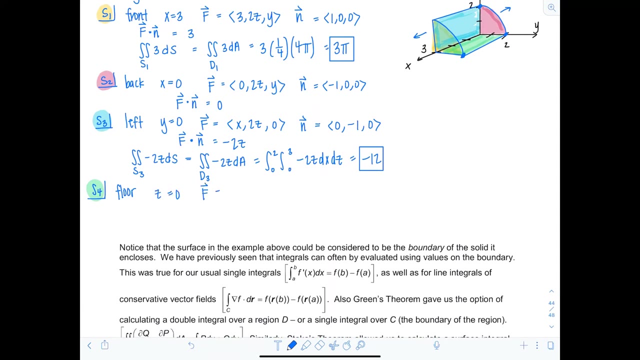 down here, determined by the portion of the xy plane Surface. 4 is the floor. Okay, so what's the equation? It's the portion of the plane z equals 0. So on that plane, my vector field, go back, substitute in 0, right for z. So you'll just. 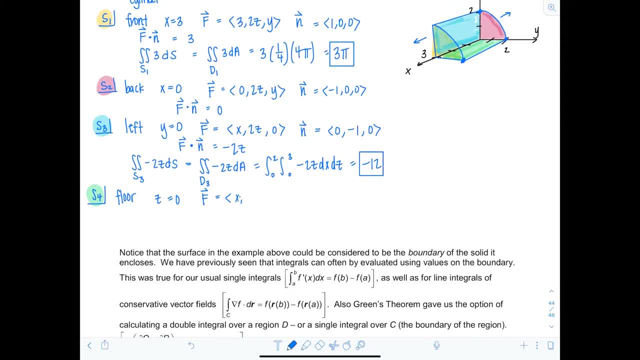 have x, 0, y. Now what's the normal vector outward from the surface at that portion of the plane? Well, it would be going to be the xy plane. So it's going to be the xy plane, So it would be. 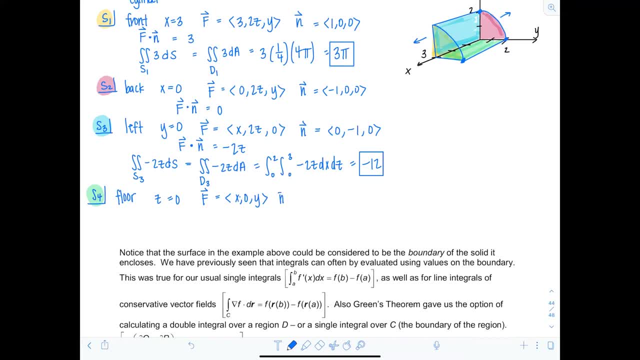 the xy plane. So it's going to be the xy plane. So it's going to be the xy plane. So it's going to going in the negative z direction. So for n we're going to use 0,, 0, negative 1,, which means 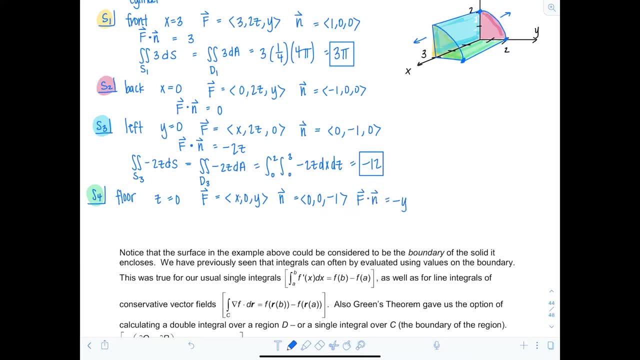 f dot n is going to be negative y. All right, very good. So then our surface integral for surface 4 would be negative y. ds That surface. I'm going to integrate it over the xy plane. So we're going to have double integral over d4, which is just that rectangle in the xy plane. 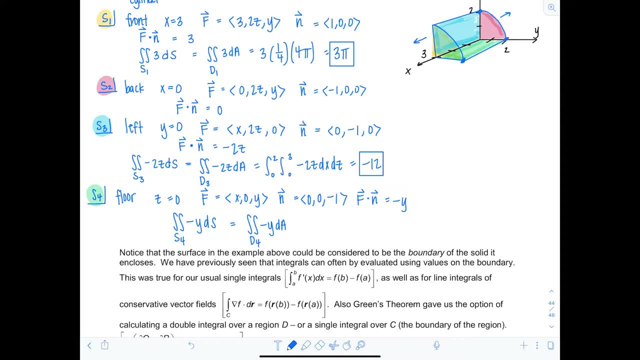 and I have negative y da, And then you could set it up. It's just as easy. if it's dx, dy or dy dx, I'll put limits for y on the outside. So that means 0 to 2 in the y direction. 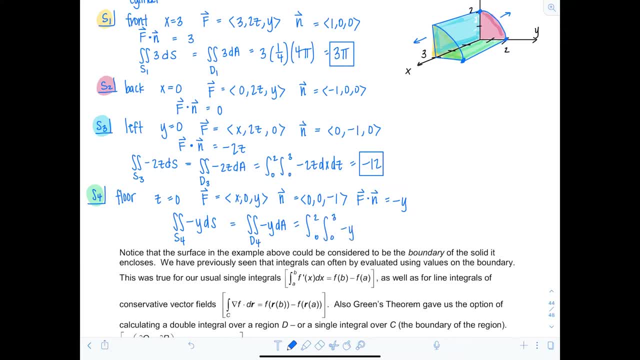 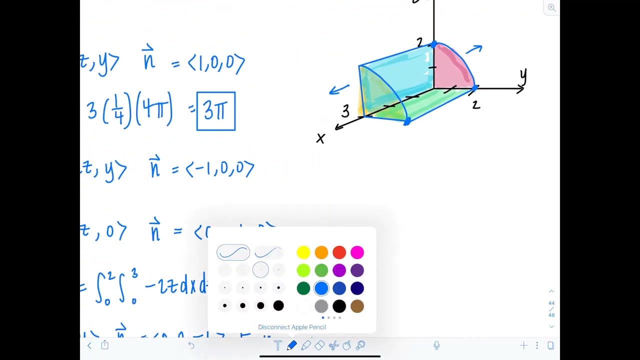 0 to 3 in the x direction. negative y, dx, dy, which is negative 6.. Okay, nice, Now there's one more surface, That's the cylinder itself. yes, Okay, so let's zoom in so we have a little more space. So surface 5: 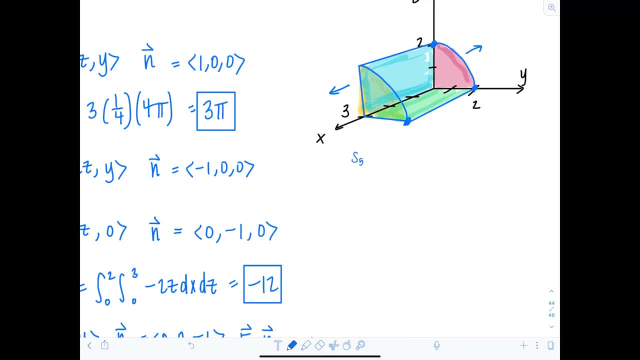 is the actual cylinder itself. I'm not going to color it in just because it's going to make a mess, but basically it's this face here. That's our fifth surface. Okay, well, what determines the equation of that surface? Well, it comes from the cylinder's. 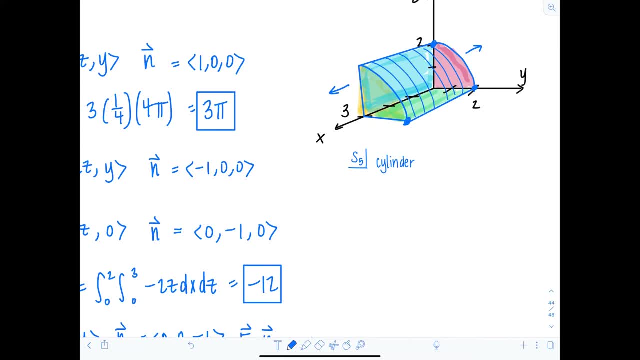 equation: y squared plus z squared equals 4, and I'm only going to solve for one of the variables and decide now: do you want to solve for y or solve for z? I think it's easier if we solve for z, because then I could integrate over the xy plane, okay, which is just like a nice little rectangle. 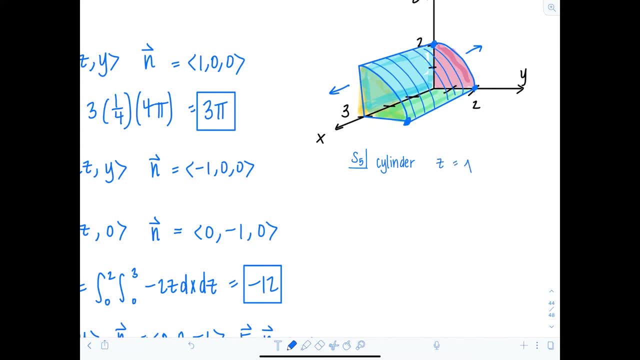 So if I solve for z, remember we're in the first octant, so I'm going to choose the positive y squared and then I'm going to substitute that in for z into my vector field. So the components are going to be x 2 times rad 4 minus y squared, and then the last component is y. 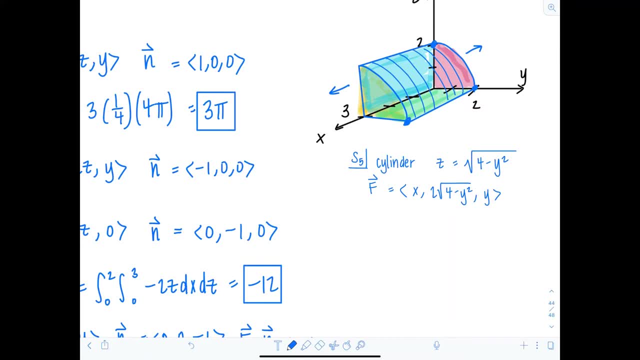 Now for our normal vector. okay, this is where it gets a little bit trickier. So just imagine you're walking on that cylinder. okay, and remember, standard orientation is outward. So if you're walking on the cylinder and you get close to the top, right here, right- and then imagine you're basically at the top now. 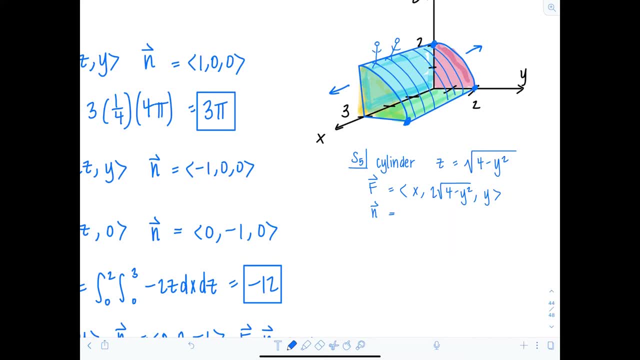 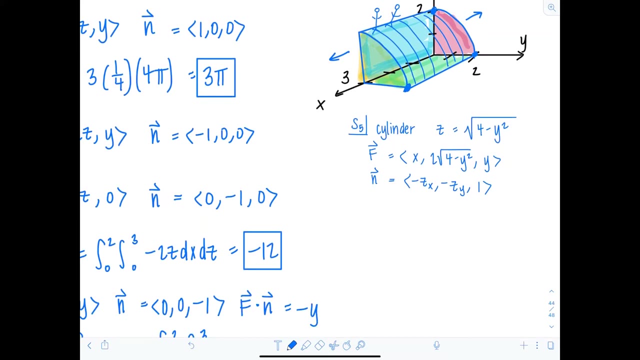 The z component would be positive 1, and so that means the other two components are going to be negative partial with respect to x, negative partial with respect to y, and then that last component's positive 1,. okay, So from here, remember always determine the sign of the constant. 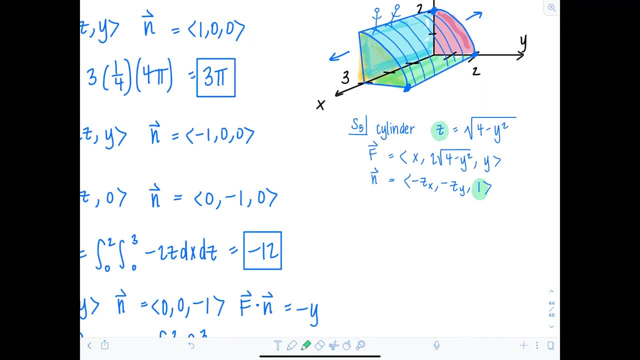 So since we have x 2 times rad 4 minus y squared, and then the last component's positive 1, had z as a function of x and y, then you figure that out. first the z component, if it's positive. 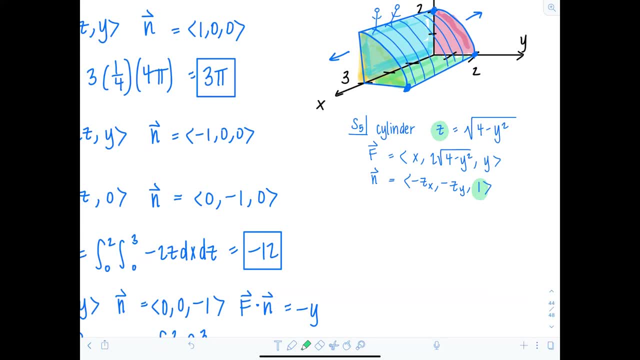 or negative, and then the other two partial derivatives have the opposite sign. All right, great. So that means, in this particular case, n will have components. well, there's no x's, so just 0, and then y over rad 4 minus y squared, and then I'm left with 1.. 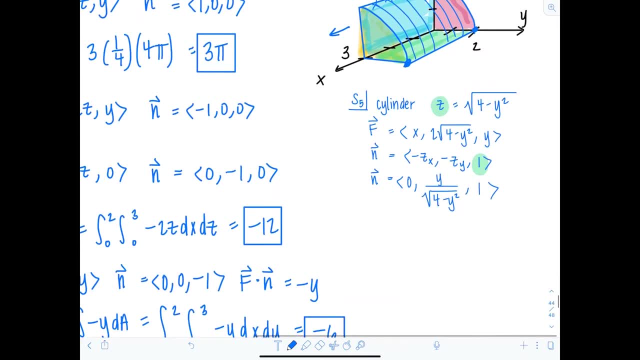 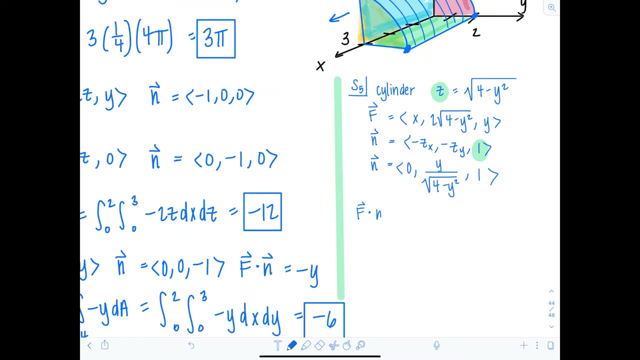 Okay, so f dot n. f dot n is going to be not so terrible. it looks worse than it is right. This is 0.. Notice here: when I take this product, the radical 4 minus y squared cancels out. 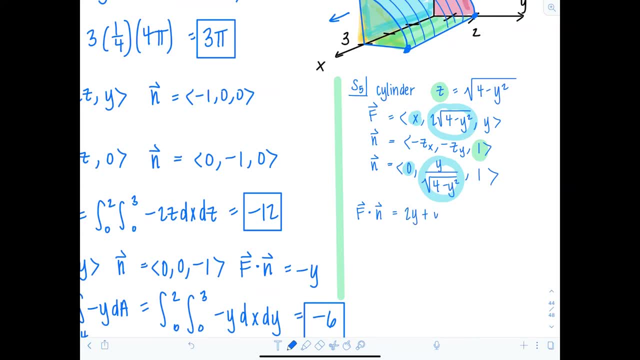 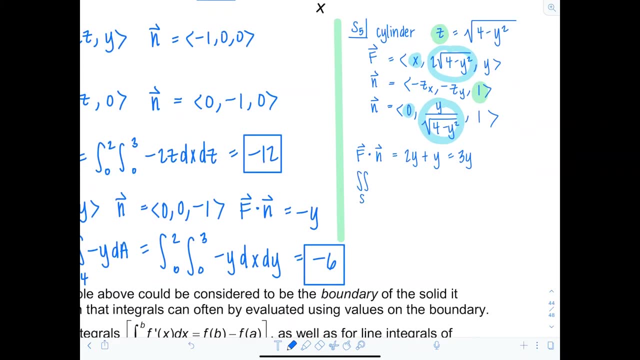 so I'm just left with 2y plus y, so 3y. Good, so now surface integral over surface 5 of 3y ds. and then, remember, we chose to solve for z, so we could just integrate this surface over the xy plane and our region. d is just this. 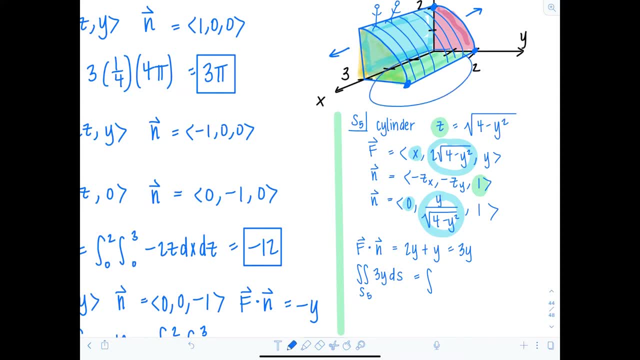 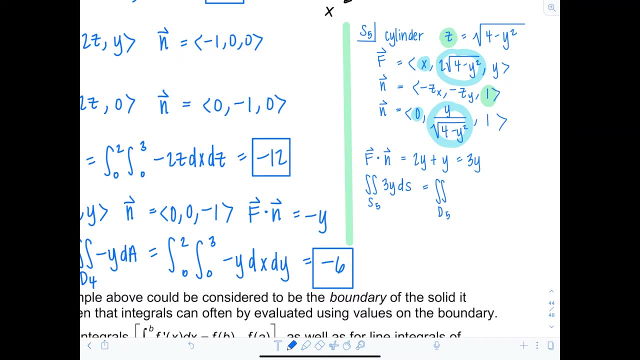 nice rectangle here. Oops, didn't mean to do that. This rectangle here, that's d. Okay, so I have double integral over d5 of 3y, dA, which is going to be limits for y, or from 0 to 2, limits for x or from 0 to 3, and then I have 3y, dy, dx. 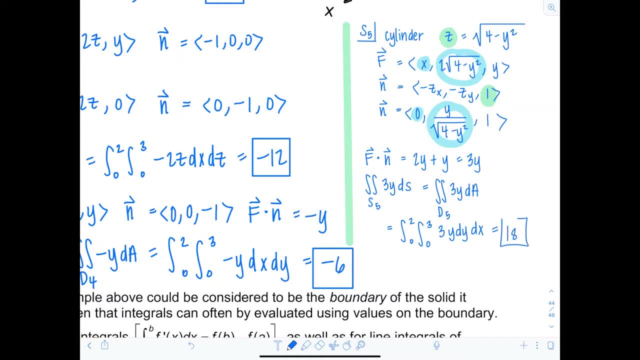 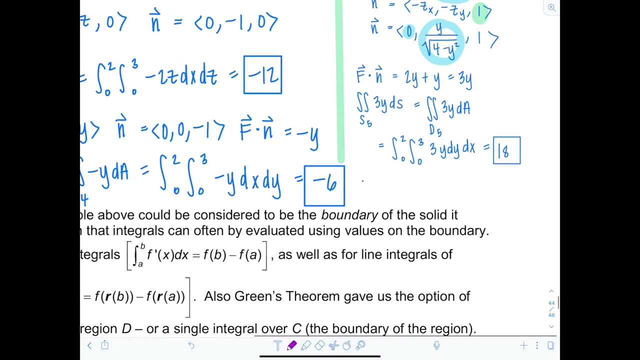 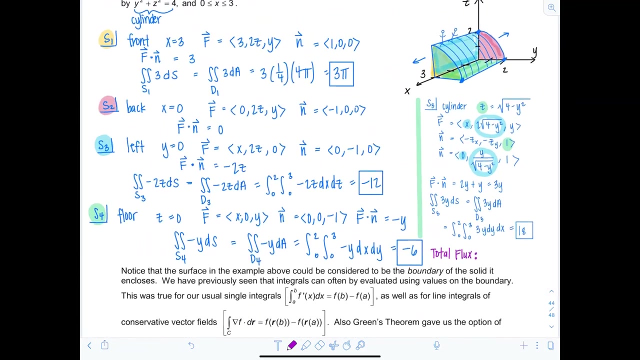 And this gives me 18.. Goodness gracious, Okay. so basically, to get the total flux, we're going to add the flux from each of the five surfaces together, And so, So what are our results? Let's see. Let's recap: We've got 3 pi. Second surface was 0.. 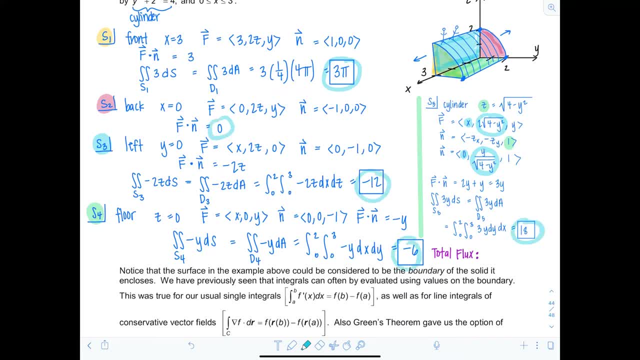 Then I have negative 12,, negative 6, and positive 18.. So those all cancel out. I'm just left with 3 pi And that's your final answer. Okay, It was tedious, but it worked. And notice that the 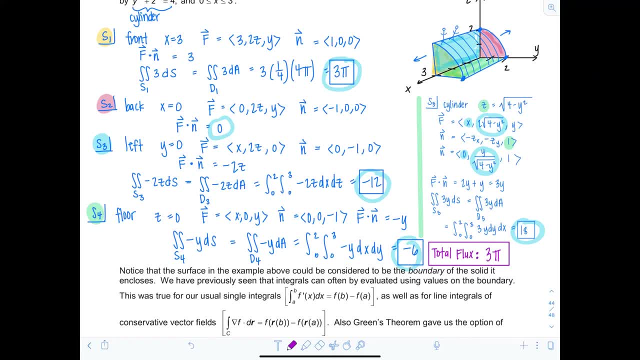 surface in the example above, could have just been considered to be the boundary of the solid that it encloses, And we've previously seen that integrals can often be evaluated only using values on the boundary, And this was true when we looked at single integrals right, Our fundamental theorem. 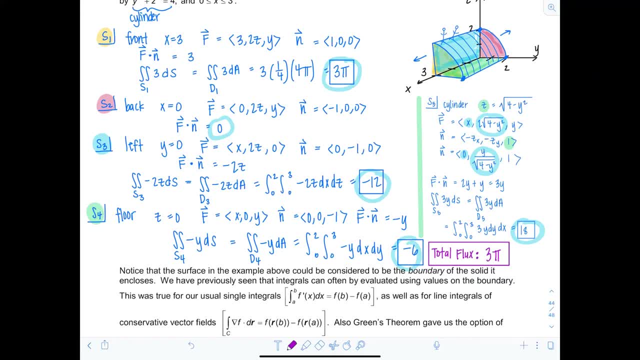 of calculus told us: if we had the definite integral from a to b of f, prime of x, dx, we just evaluated the antiderivative at the endpoints of the interval. This was also true for line integrals. So if we had the definite integral from a to b of f, prime of x, dx, we just evaluated. 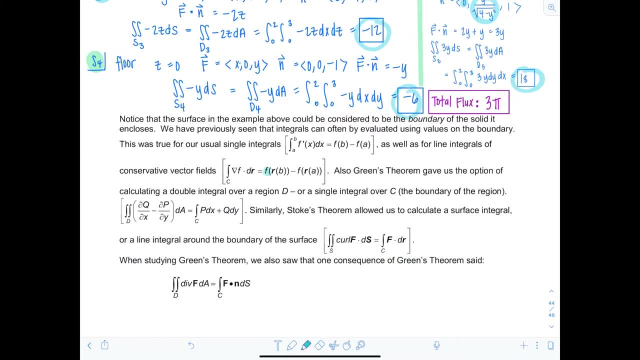 the antiderivative at the endpoints of the interval. This was also true for line integrals of conservative vector fields. Remember, we just had to find the potential function for our conservative vector field and then evaluate it at the starting and stopping point of our curve. 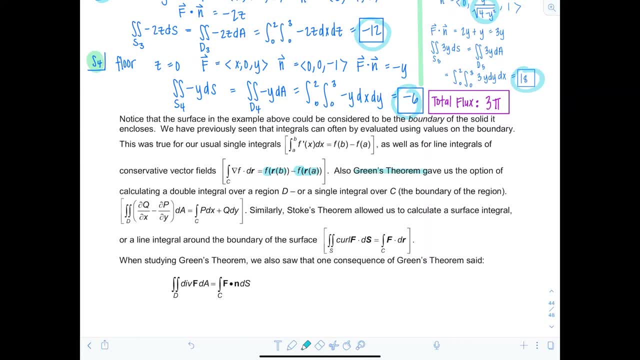 And then Green's theorem. don't forget about Green's theorem. it gave us the option of calculating a double integral over a region d. Or you could do a single integral over c, where c was the boundary of the region d. So here's Green's theorem. 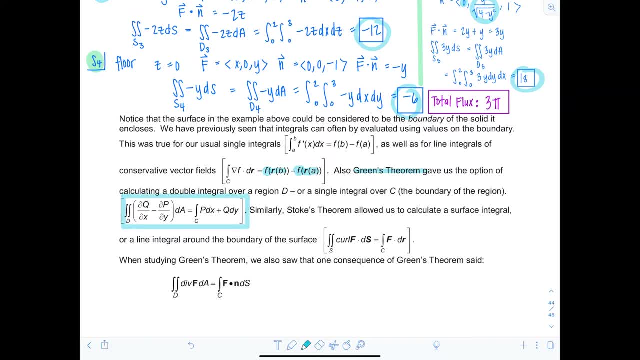 Remember Green's theorem we used to find work. Similarly, Stokes' theorem allowed us to calculate a surface integral or a line integral around the boundary of the surface, And again this integral helped us evaluate work. Now, when we were studying Green's theorem, we also saw that one. 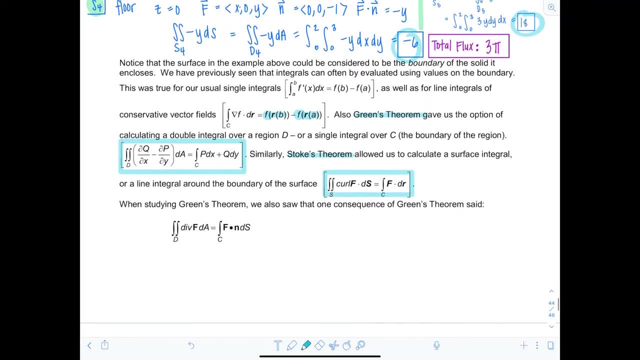 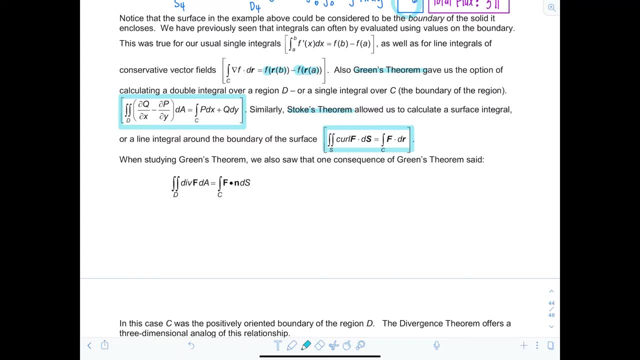 consequence of Green's theorem stated that the double integral over the region d of the divergence of f- dA was equal to the line integral over c, where c is the boundary of d of f dotted with n? ds. And remember this quantity here has a different interpretation that doesn't represent work. 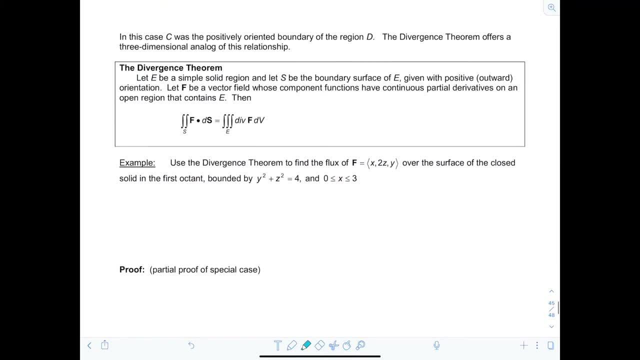 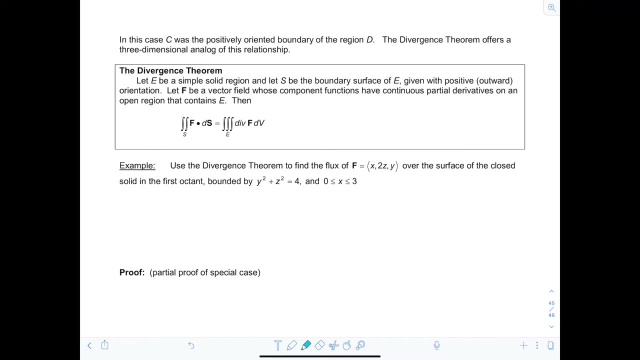 Now, when we were looking at Green's theorem, c was a positively oriented boundary of the region d and we were only working in the xy plane. But now we want to work in 3-space, and so the divergence theorem offers us a three-dimensional analog of this relationship, and it states the following: 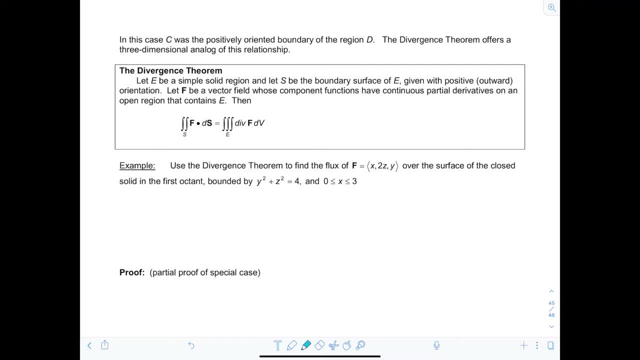 So let E be a simple, solid region, let S be the boundary surface of E, given with positive outward orientation, and F is a vector field whose component functions have continuous partial derivatives. on an open region that contains d, Then the surface integral over s of S dot dA is not the boundary. or the gradient surface, but it input the boundary E over P, so it Unter assaults the appropriate boundary and filters negative của electric induction On an open region with partial derivative viens against E. So we run this simulation again. So g measure b tells the surface integral over S of E. 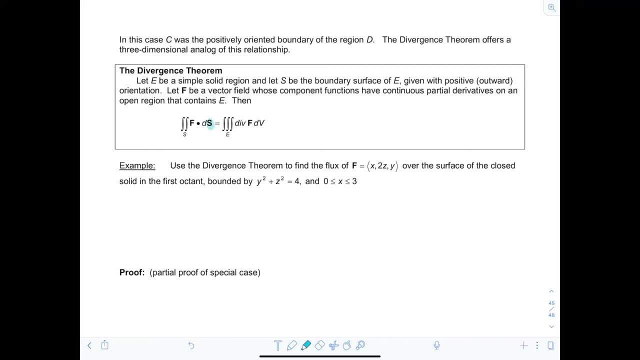 edge with the entire surface And where g pushing is coming from as piece of the integral. So let g be the boundary surface. dot ds and notice this: s is a vector. quantity is equal to the triple integral over e of the divergence of f- dv. And just to reiterate, what does this integral represent? This is flux. 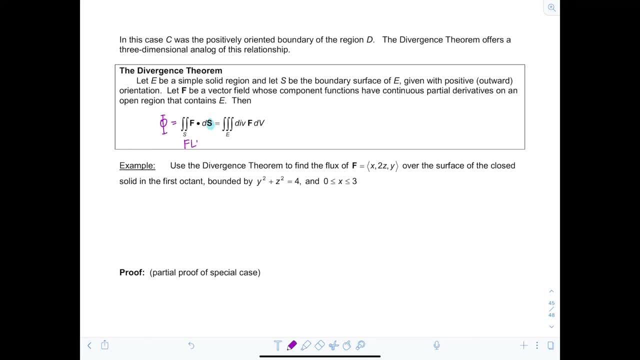 This is flux. Okay, so Stokes' theorem we used to evaluate work. The difference was we had curl of f, dot ds and in this case, for flux, you don't have the curl. Good, All right, so Stokes' theorem. 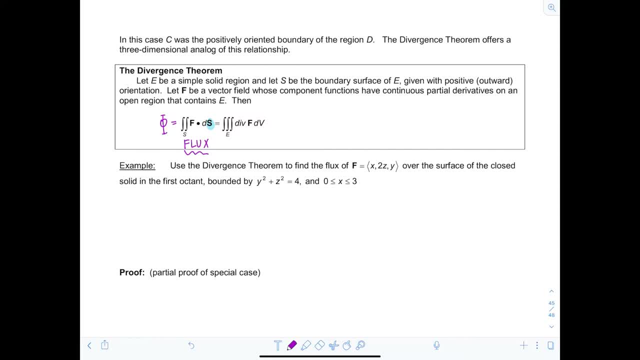 you do line integrals, relate them to surface integrals. Divergence theorem: you're working with flux. you do triple integrals and relate them to surface integrals. So let's see just how snazzy this divergence theorem is. We're going to use it to find the flux of the vector. 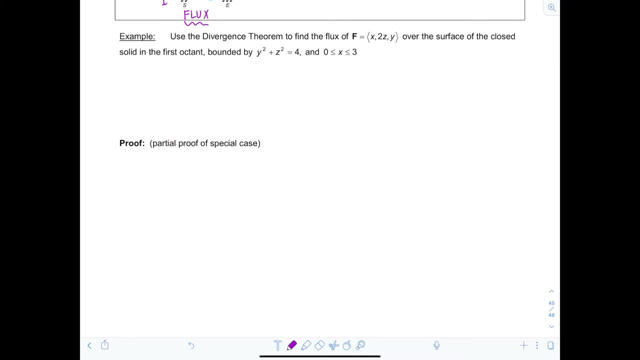 field from the previous example that we just did: over the surface Of the closed solid in the first octant, bounded by y squared plus z squared equals four x between zero and three. So using the divergence theorem, I'm actually just going to evaluate. 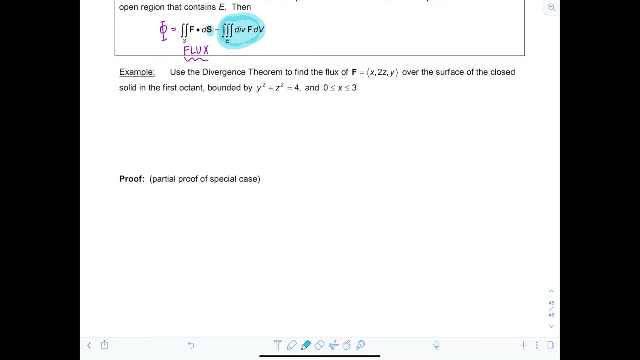 a triple integral over the solid e. so I need the divergence of f. So divergence of f, if you'll remember, here's pqr, right, You just take the partial derivative of each component with respect to the corresponding variable and add them together. So I'm going to take partial. 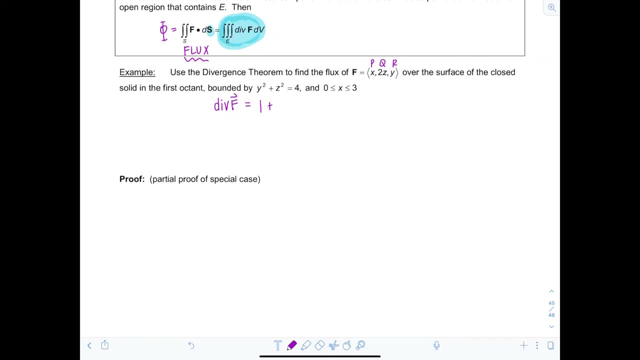 derivative of x with respect to x, that's pqr, and I'm going to take the partial derivative of x with the corresponding variable and add them together. So I'm going to take partial derivative of x with one. Partial derivative of 2z with respect to y- that's just zero, And partial derivative of y with 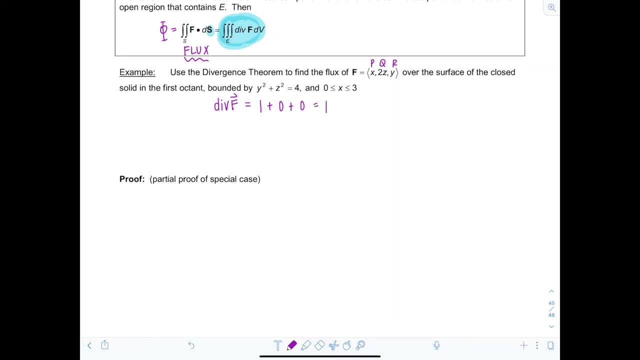 respect to z is zero also, so this is one That means the flux is equal to the triple integral over e of one dv. And remember, if you have a triple integral of just dv, that represents the volume of the solid over which you're integrating. 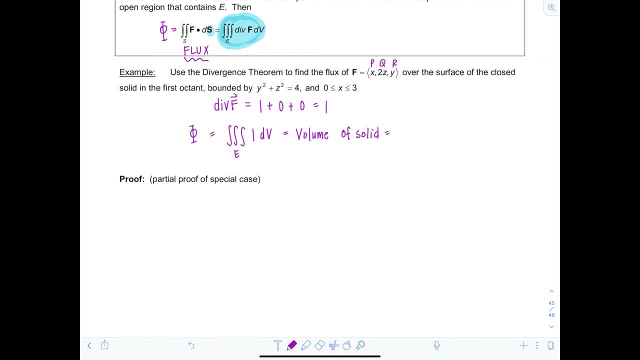 And remember, this solid is just a quarter of a cylinder, And so we could set up an integral if we wanted, or I know how to find the area or, excuse me, the volume of a cylinder: It's just pi r squared h. So this would be pi times 2 squared times h, which is 3.. Okay, so the one. 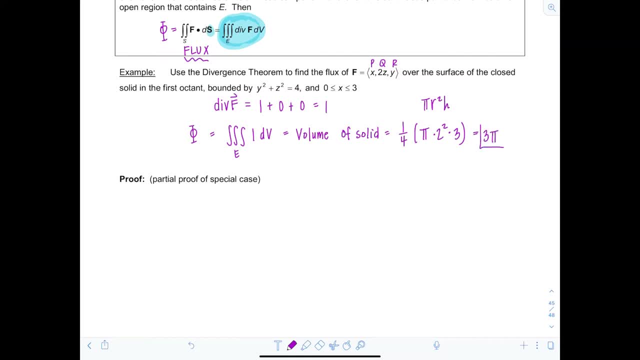 fourth of 2 squared are going to cancel and I just have 3 pi left over. And that's it. Wasn't that much less painful Than setting up 5 surface integrals? Okay, well, let's look at a proof. And we're not going to prove. 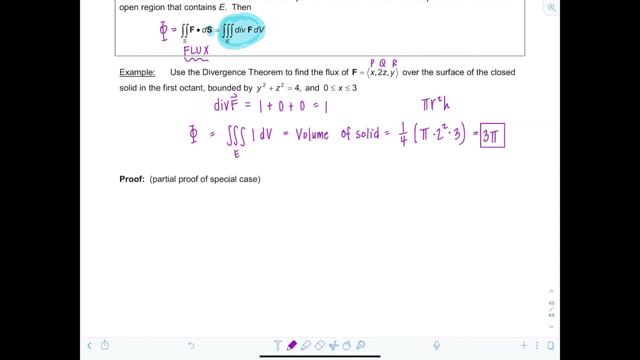 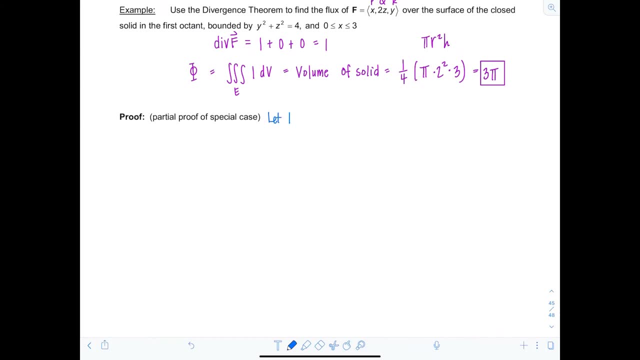 the divergence theorem. in completion, We're just going to do a partial proof of a special case. Okay, so to begin, we're going to assume we have a vector field F with components p, q and r, and it's going to satisfy all the necessary conditions. They have continuous partial derivatives on an. 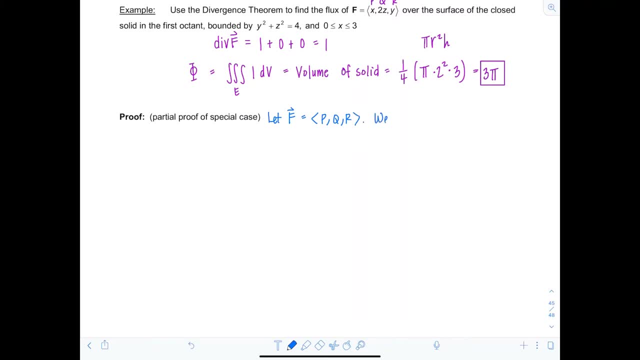 open region. Okay, so we're going to assume we have a vector field F that contains the solid E, And what we want to do is show that the surface integral over S of F dot n dS- remember, when this is not a vector quantity, that's because I've replaced S, the vector, with F dot n dS- This is equal to the triple integral over E of the divergence of F? dV. 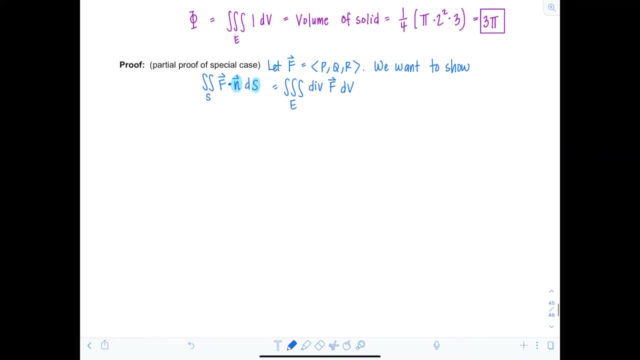 okay, Okay. Well, what is this equivalent to? I just Zak tales. I just defined my vector field to have components p, q and r, So double integral over S of p, q, r dotted with n dS. So I just substituted pq r. 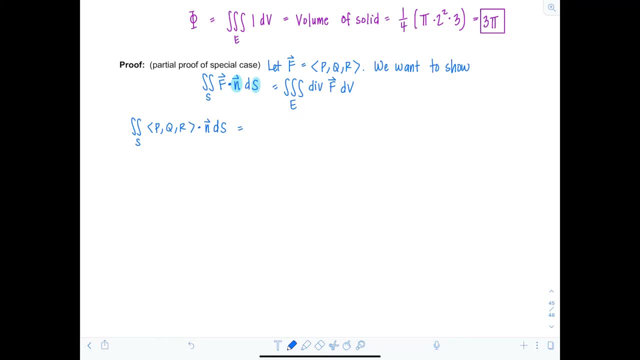 and for f is equal to: And I'm just going to take this dot product right now. So I have surface integral over S of p. i hat dot all of these items, dot p. i hat dot all of these things. 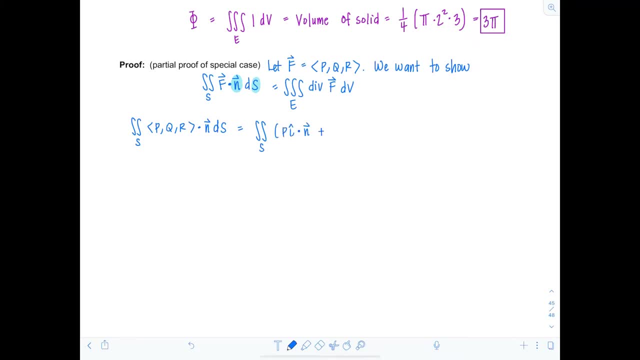 dot p. i hat dot all of these things. dot p. i hat dot all of these things with n plus q j hat dotted with n- I'm just switching my notation, okay- plus r k hat dotted with n? ds. And what we're going to do right now is we'll show that this actually equals. 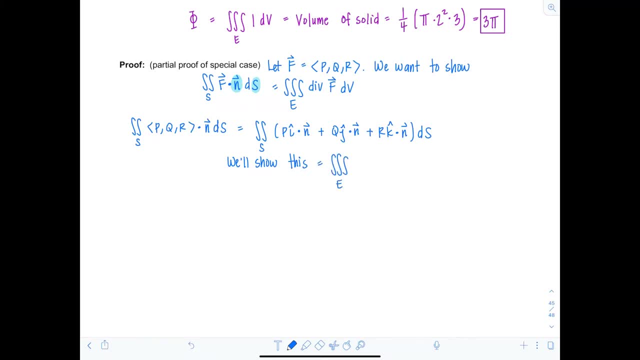 the triple integral over e, and then, instead of divergence of f, I'm actually going to write out that would be del p, del x plus del q, del y plus del r, del z, dv. okay, How am I going to show this In order for these two integrals to be equal? 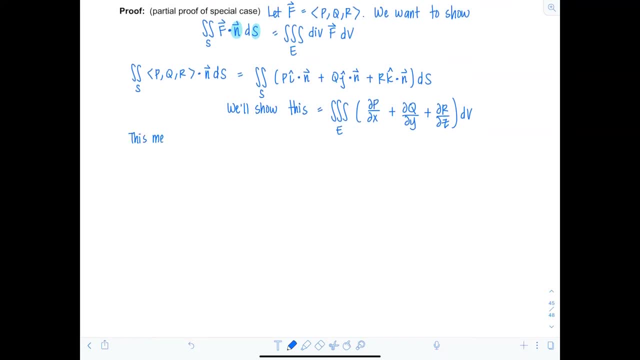 think about what it would mean. So this means that our surface integral of p i hat dotted with n ds, would need to equal our triple integral over e of del p, del x, dv. I mean those are the only parts of each of the integrals that 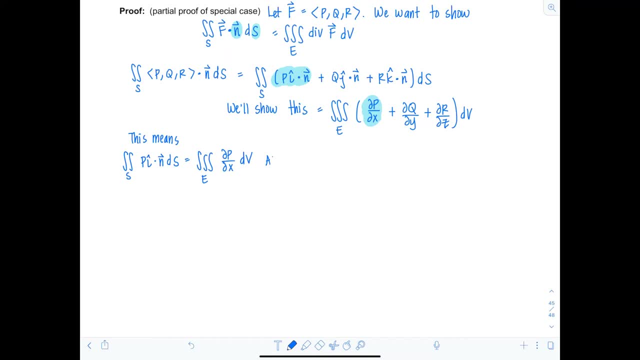 involve p right And our surface integral of q j hat dotted with n? ds would need to equal the triple integral over e of del q del y dv, And surface integral of r k hat dot n ds would need to equal triple integral over e of del r del z dv. 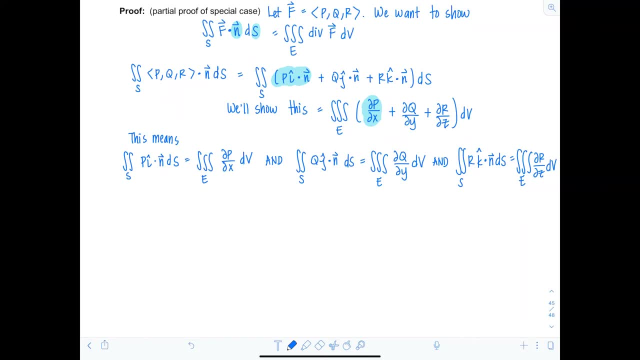 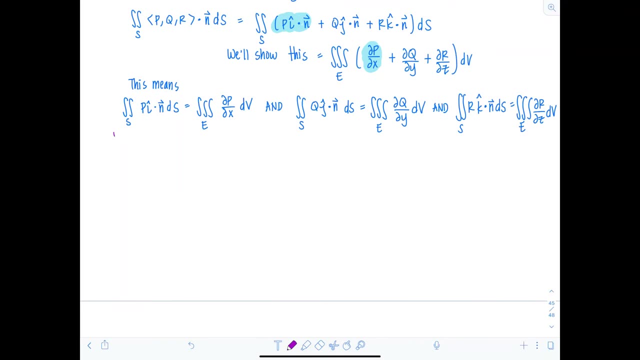 So if I could show all three of these equalities then I'll have proven what we needed. I'm just going to do part of it. This is a partial proof. So right now we will prove that the surface integral of p i hat dotted with n? ds would equal the total integral over e of del r, del z? dv And. 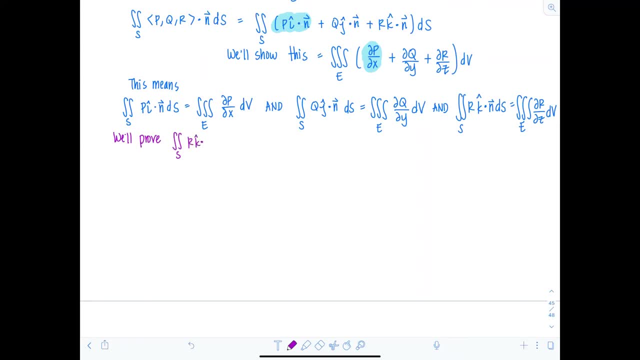 integral of r k hat dot n d? s. just that last one is equal to the triple integral over e of del r del z d v. Okay, so we're just going to focus on this Now. I said we're doing a partial. 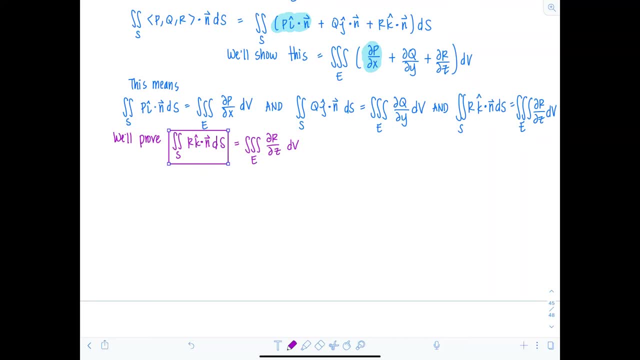 proof? yes, because we're only working on a third of it, basically, and we're working on a special case. So we're going to assume our solid e can be bounded with three surfaces, okay, and say this is surface one. z can be expressed as a function of x and y. That's what I'm assuming. 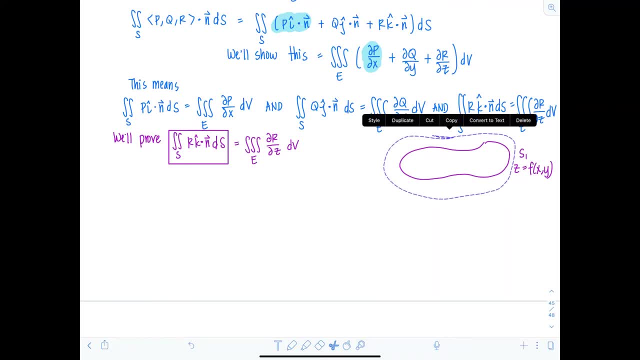 about this surface Okay, and then here's surface two. It's not necessarily identical, but both of them can be evaluated over the same region, d in the xy plane. Okay, it's kind of a bold assumption. So there's surface two, there's surface one, and then surface three is perpendicular. 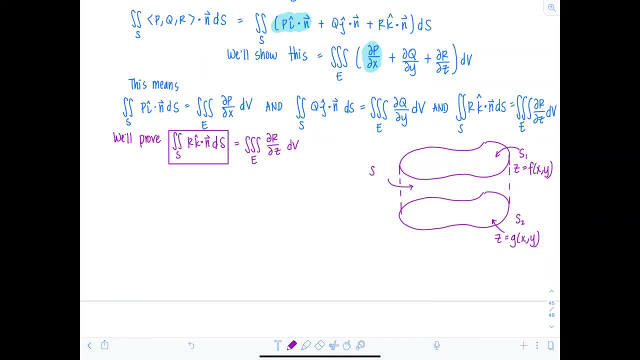 to the xy plane. Okay, very good. So surface three is vertical. So if I want its normal vector, it's going to be a horizontal vector right Normal outward, Just imagine be something like this right Outward. What does that mean? That means its z component is zero. 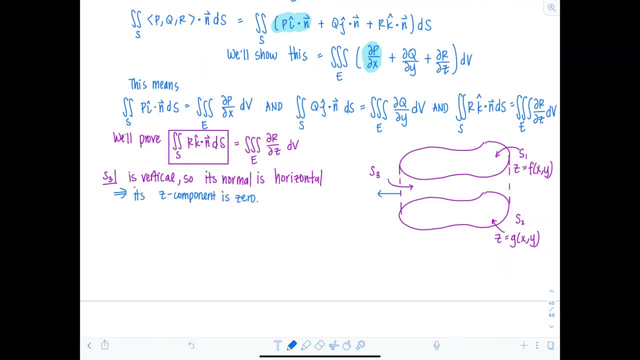 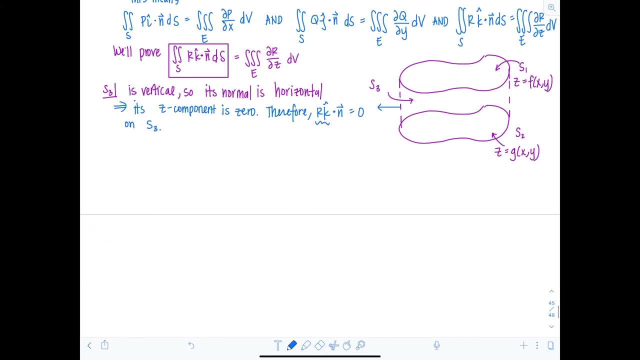 Zero or rk hat dotted with n for that surface would equal zero, right, Because this is only in the z component on S3.. All right, what about surface one? Shall we shade it in? Do we need some shading? Why not? 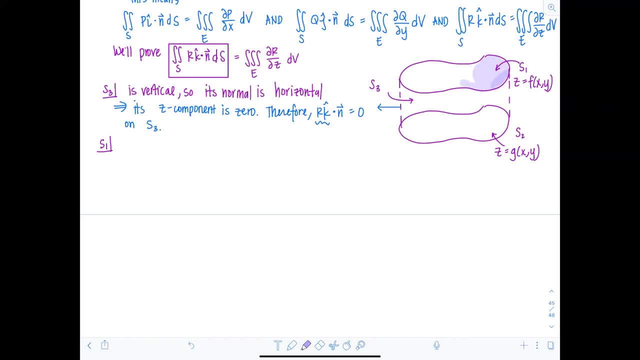 So here's surface one. Okay, let's think about which way the normal vector is going to go. So standard positive orientations: outward, upward. Imagine you're walking on surface one Here you are having a grand old time. Outward is up in this case. 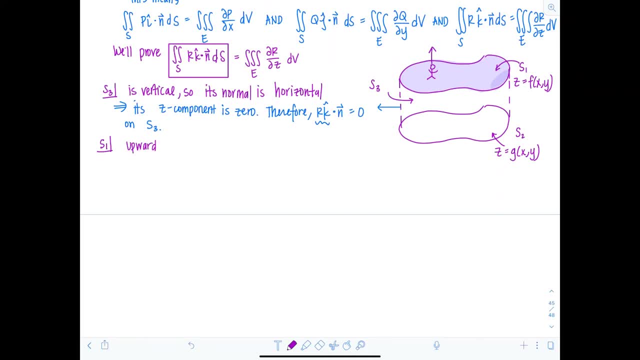 Okay, upward. So what does that mean? That means the z component is going to be positive And surface one. I can express as a function of x and y. So the normal vector, If I know the z component is going to be positive one. 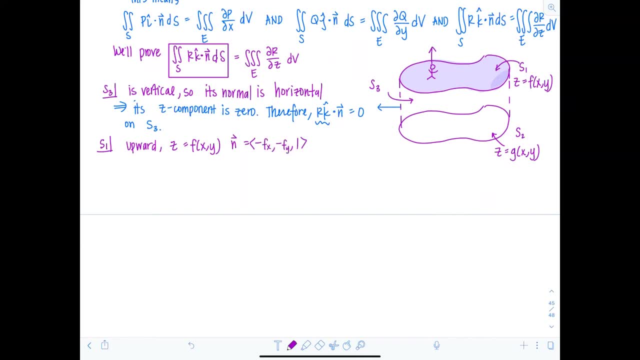 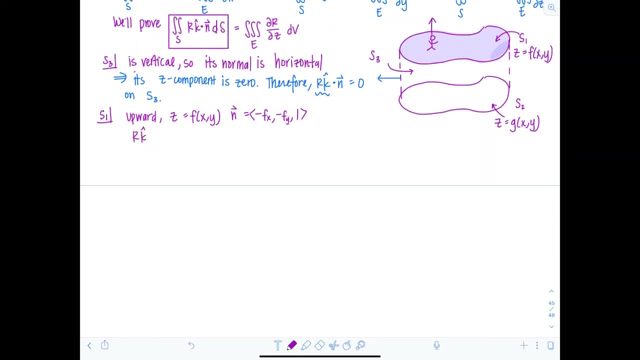 that means the first two components are negative, partial with respect to x, negative partial with respect to y. So let's go ahead and find rk hat and dot it with n. Okay, I don't have a formula for what r is, but rk hat would just have components 0,, 0, and then whatever r is. 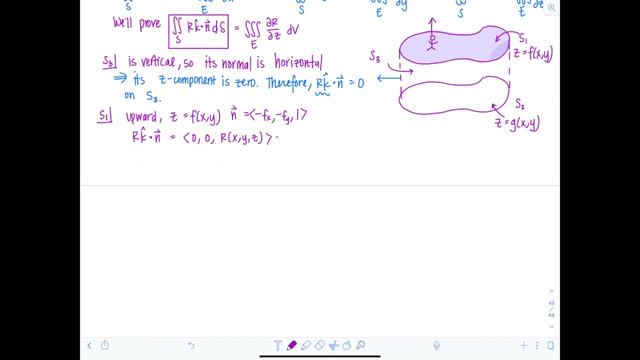 It's a function of x, y and z, And then if I dot that with the normal on surface, one negative partial with respect to x, negative partial with respect to y, positive one, And then when you take the dot product, you just get r of x, y, z. 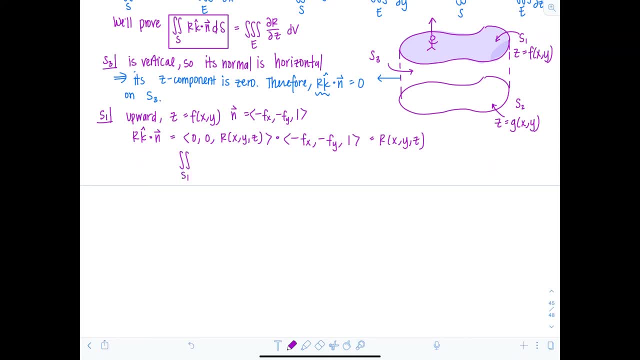 So let's see, I'm going to find the flux, I'm going to evaluate the surface integral on surface one, rk, hat, dot, n, d, s- And I'm going to integrate this surface over some domain d in the x y plane. 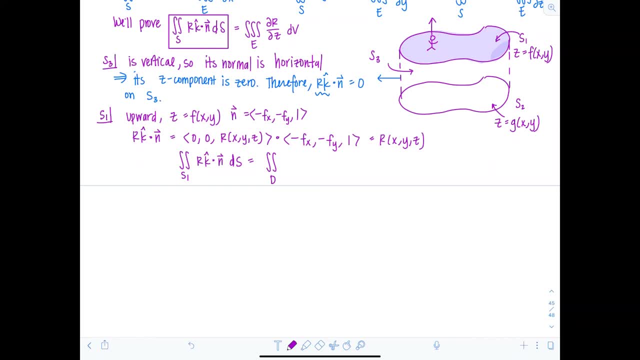 And I know that this dot product right here is equal to r of x y z, So I could write that as r of x- y and then we're on surface one. So on surface one, z is f of x y, right. 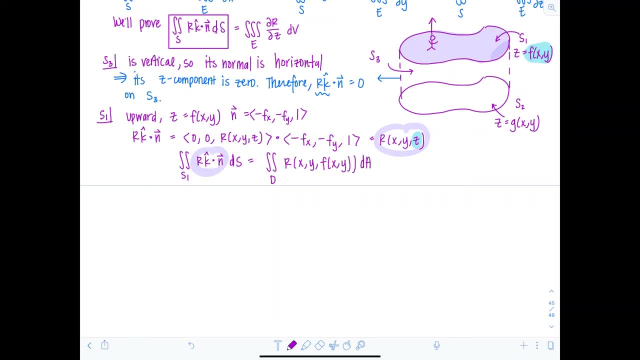 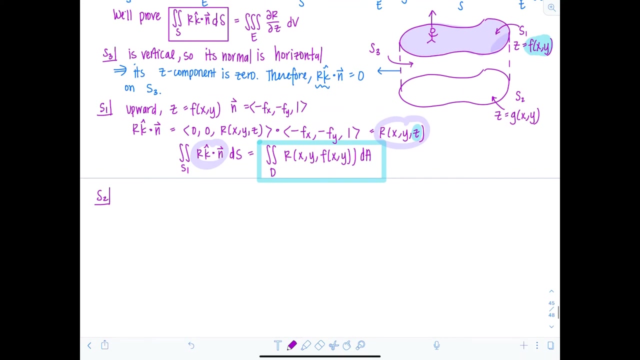 Da. Okay, put that on the back burner, on hold, Shall we box it. Yeah, Exciting stuff. Now we move on to surface two. Time for surface two, What would be the orientation for our normal vector? Remember, it's going outward. 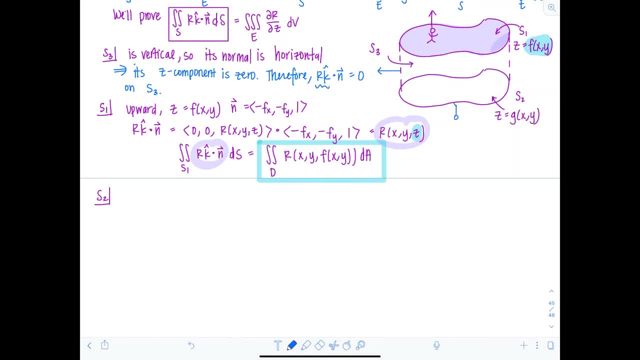 So you're a person walking on the surface, Your head is pointing in the negative z direction. So outward orientation in this case would be downward, Which means on that surface z is a function g of x and y And the normal vector would have negative one. yes, 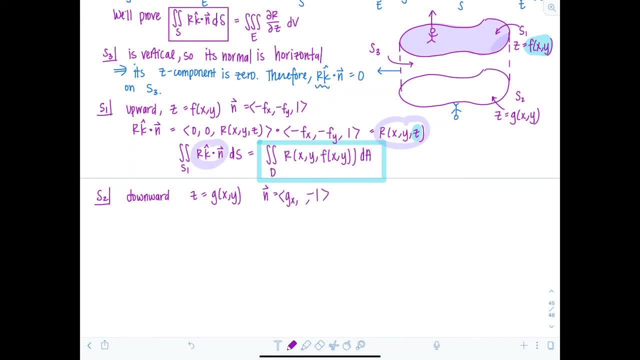 For the z component. So that means the x component would be the partial with respect to x- Let's skip this over. And then the y component would be partial with respect to y. Always the opposite signs of the constant One or negative one. 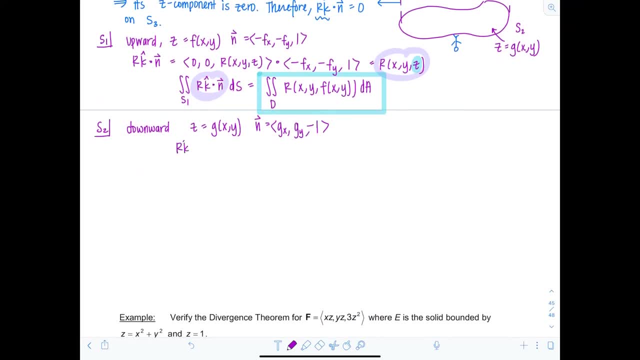 Okay. So then now let's figure out r, k hat dotted with n. on that surface It would be zero, zero r of x, y, z, dotted with partial with respect to x, partial with respect to y, negative one. 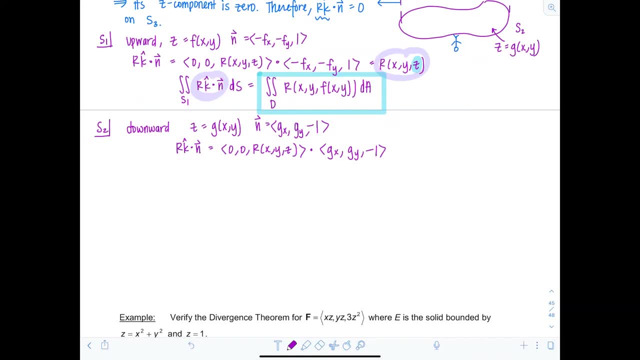 Remember, I'm using g because we're on surface two And I'm left with negative r of x- y and then, just like last time, I can replace z with g of x- y. Okay, so now, if I find the flex, I'm going to evaluate the surface integral for that. 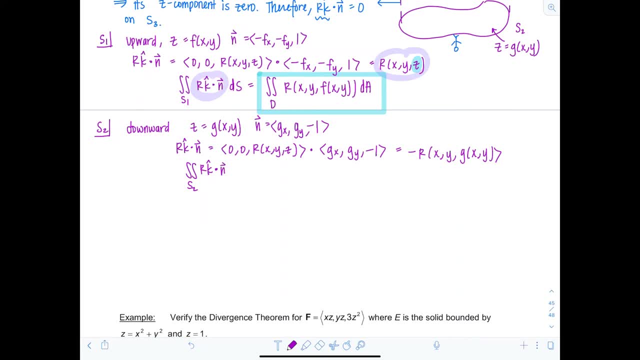 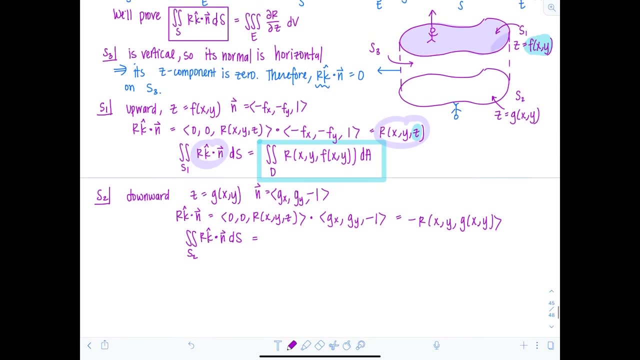 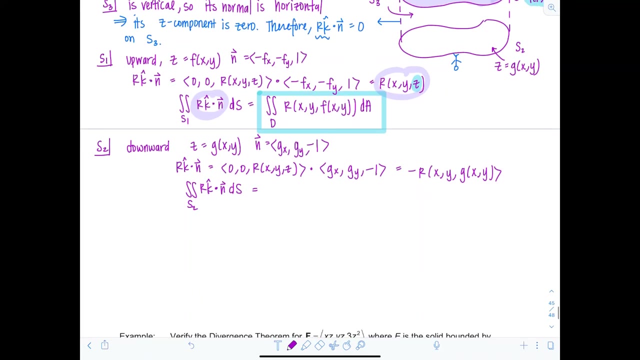 second surface of r k hat dot n ds, which is equal to. and then here's you know our oversimplification. We're assuming it's going to be the same region that I can integrate over in the xy plane. So this is the same d from the previous integral for surface one. 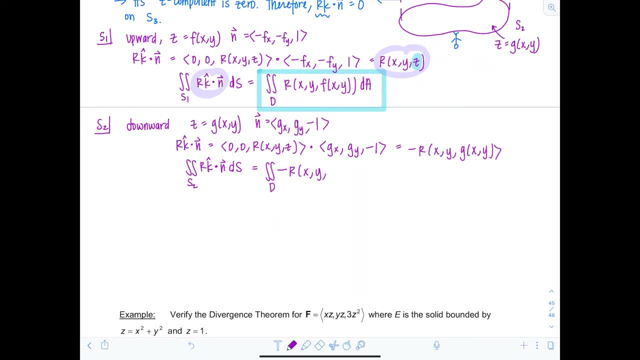 Of negative r, R of x, y and then g of x, y, dA. Okay so, if I need to put it all together, the total flux, we're just going to add the result from the three surface integrals. 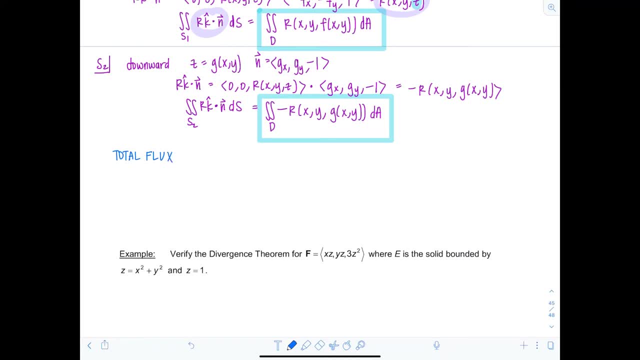 So total flux, We have zero from the first one, From surface three, plus these two which, since d is the same, I can combine them into one integral of r of x y, s of x y, minus r of x y, g of x y, dA. 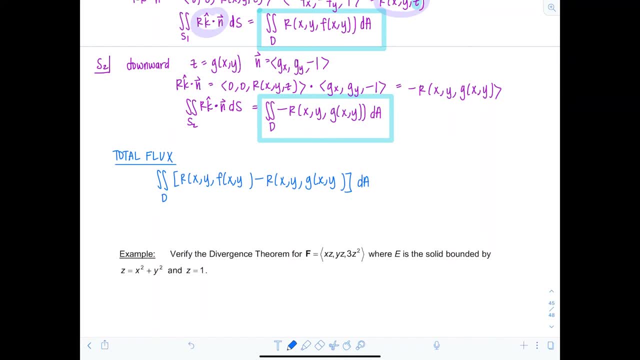 Ooh, now think about this. Doesn't this remind you of something like when you evaluate an antiderivative at its endpoints, Which means I could rewrite this. Okay, So I could rewrite this as double integral of antiderivative, with limits g of x, y, f. 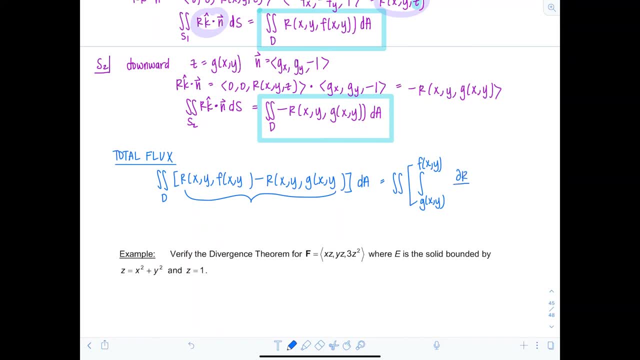 of x y del r del z dz. Yes, Because if you were to anti-differentiate del r del z with respect to z, you would just get back r of x y, And then you would substitute in f of x y for the other derivative. 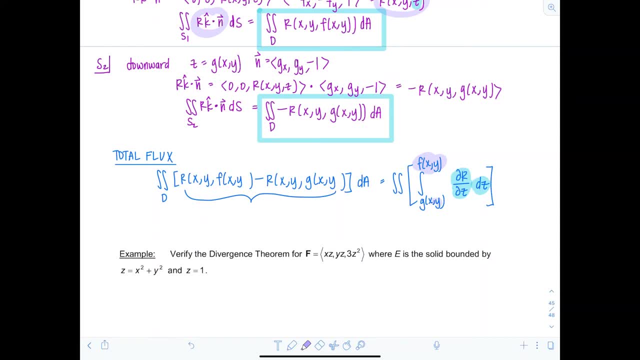 So f of x- y for the upper limit where z goes, And g of x- y for the lower limit where z goes, And I'm missing a parenthesis here. Oh, my goodness, So sorry, And I'm needing a dA. 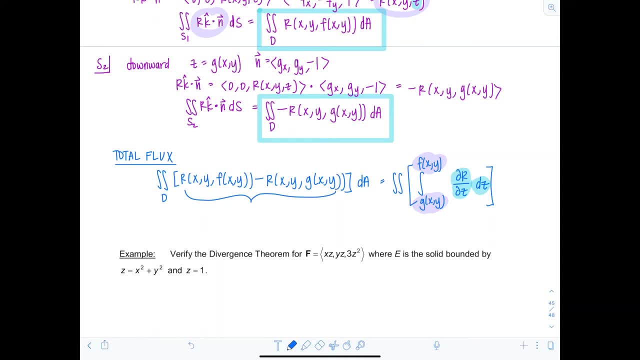 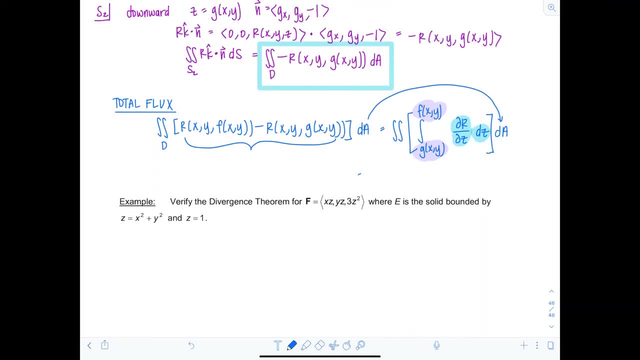 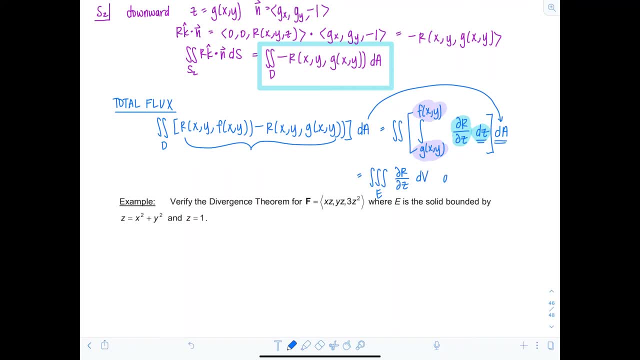 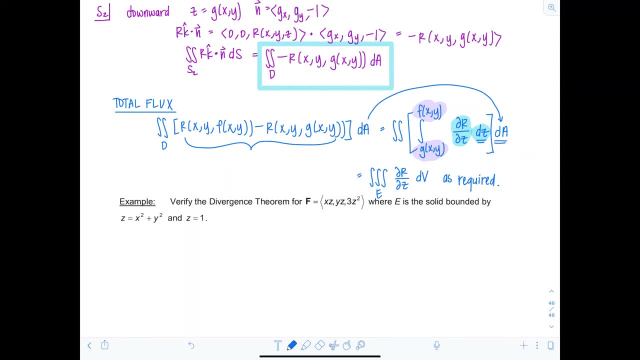 All right, And now I need to do the type shift Posted So I heat are here with me, All right, So deep-script needed damages. Where are we? How do you divide these? Oh oldies, tell me aboutvable balances. 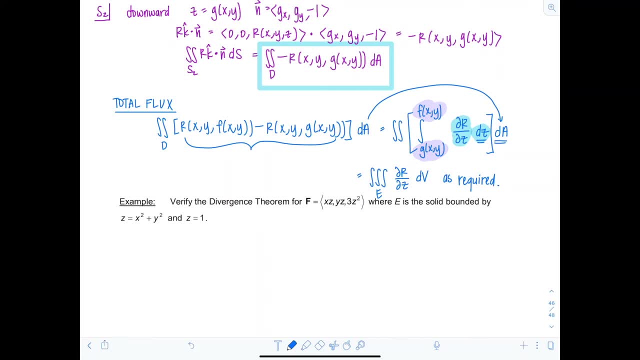 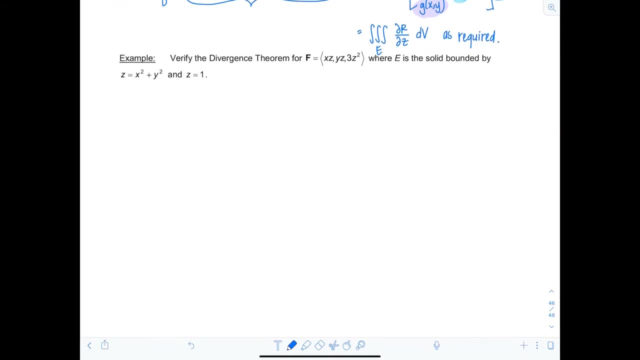 Right, Okay, Good. So this is really an interesting trade off to write. Let me add them all, Alright. So let's see, Oh gosh, solid bounded by z equals x squared plus y squared, and z equals 1.. So just to be clear. 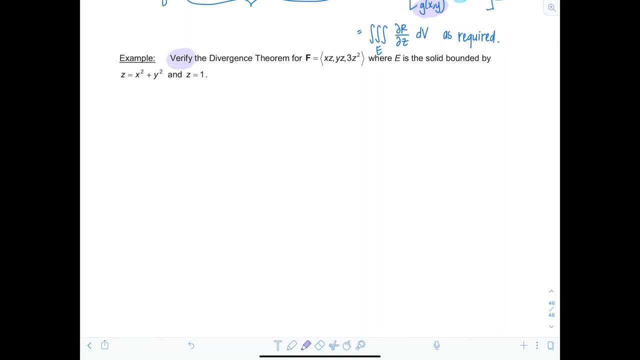 they're asking us to verify the divergence theorem. So we have to evaluate the flux as a triple integral over the solid E, and then also as a surface integral, or however many surface integrals it may take. Let's draw what's going on. Okay, E is the solid bounded by z equals x. 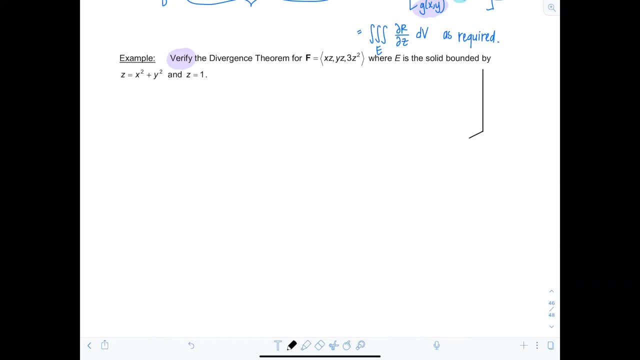 squared plus y squared, That's a paraboloid opening upward, sitting at the origin, and then z equals 1 is a plane. Hopefully at this point in our calculus career you can just graph this thing right. Okay, so here's our paraboloid, and then it's bounded by the plane z equals 1.. 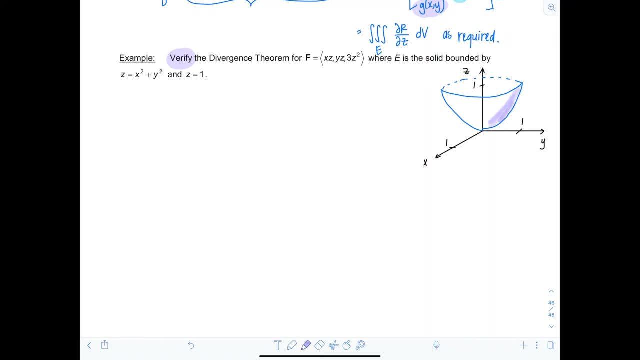 So we've got this portion, this surface here on the outside, And then we've got the plane z equals 1, that portion of it bounding the solid as well. Okay, so let's do the triple integral first. Usually that's easier. Okay, so we'll figure out here. 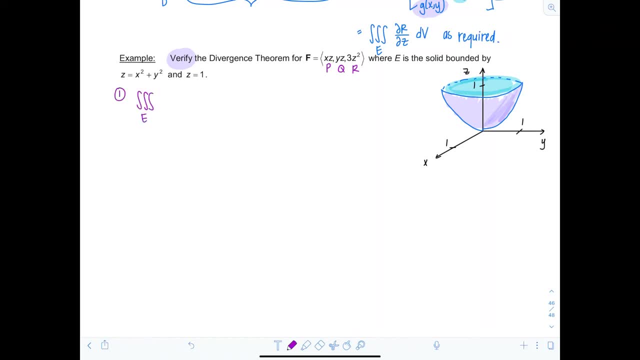 the flux by using the triple integral over E, Of the divergence of f, dv. Okay, so I need the divergence of f, So partial, with respect to x of xz. that's just z, Second component, z, Last component, 6z. 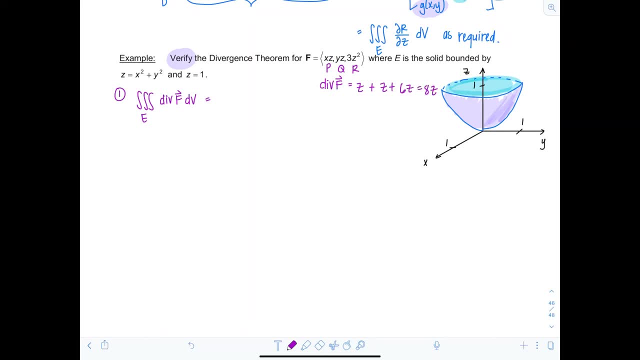 So that's 8z. All right, now, how do you want to set up a triple integral for the solid E? Well, I think the best idea would be to use a triple integral over z. You can use cylindrical coordinates, right, So I could integrate for the base region. 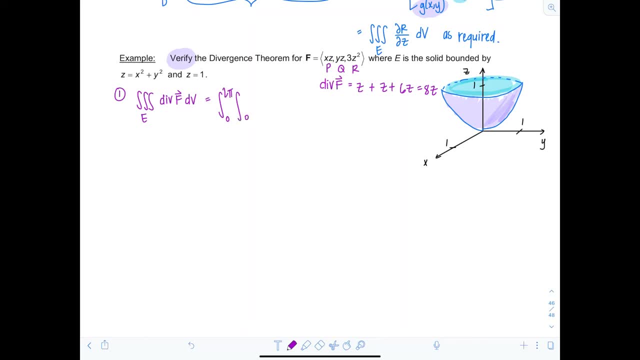 It would go from 0 to 2pi for theta, 0 to 1 for r And then my limits for z, be careful. So z starts at the paraboloid and it ends at the plane. z equals 1.. So the limits. 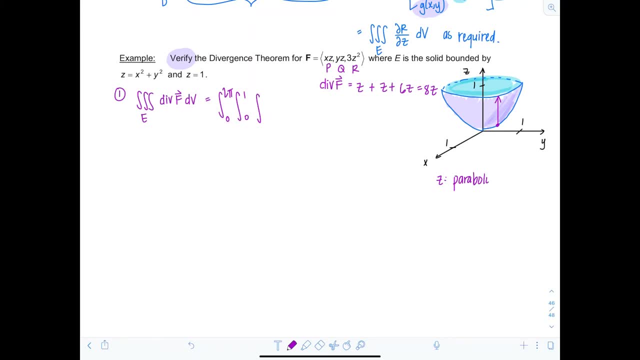 I'll write that out. z goes from paraboloid to 1. So the paraboloid's equation is x squared plus y squared. But remember we're in cylindrical coordinates, So that's going to be r squared to 1.. And then the divergence of f: we found to be 8z, So I'll leave it out there. 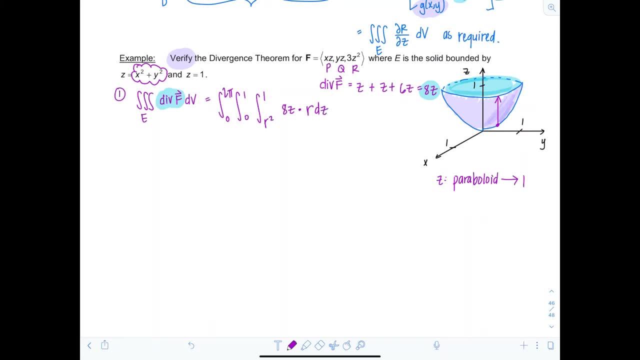 And then dv in cylindrical coordinates is r, dz, dr, d, theta, All right. and then this you can easily show is 8pi over 3. Pretty relaxing little integral. Now we have to verify the divergence theorem, So I'm going to find the flex again. 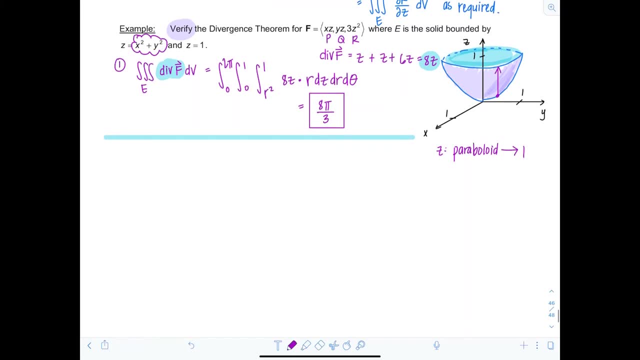 this time using surface integrals. If I'm using surface integrals, I need two of them. Is that clear? What are the two surfaces? Well, I have the paraboloid as well as that disc that's bounding it on the top, So I need f dot n? ds, So surface one. 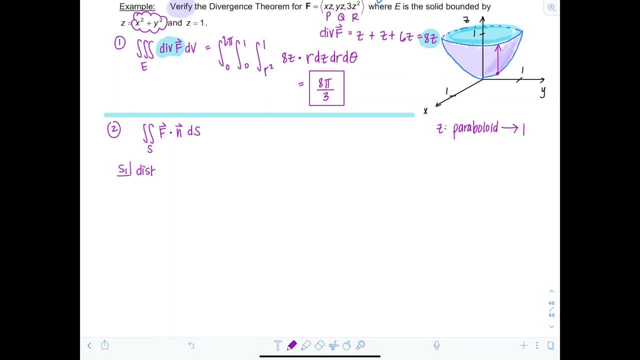 let's just do the disc at the top. Okay, surface one's the disc. So what is the equation that determines surface one? Well, it's z equals one. And remember, I'm going to substitute that in for z in my vector field, So I'll have x, y and 3.. 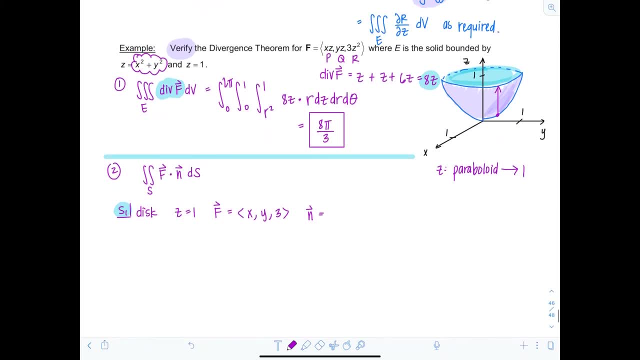 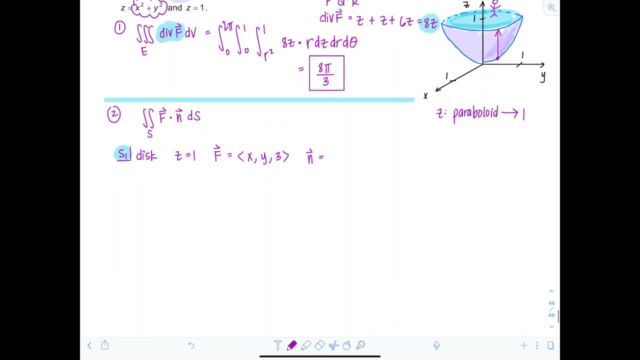 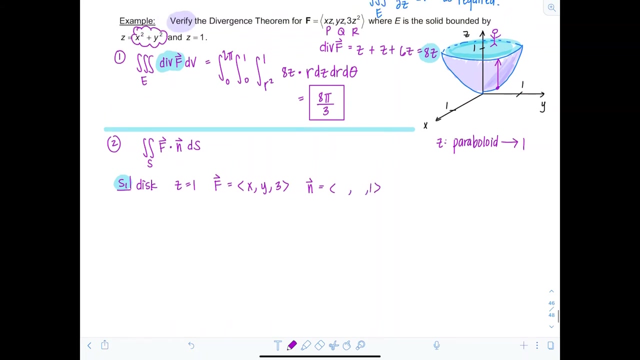 Okay, what's the orientation of my normal vector? Remember, it's outward, So you just think I'm standing here. which way is my head pointing? z is going to be positive, Okay. so once you know z is positive one, then you take your partial derivatives And this would be negative partial. 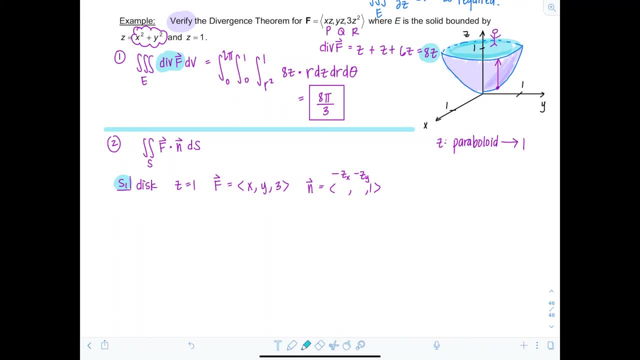 with respect to x, negative partial. with respect to y. Well, z is just equal to one, So both of those are going to be zero, Or maybe you could just tell by looking: it's going to be 001.. Bravo. And then I need f dotted with n, And that's just going to give me three. 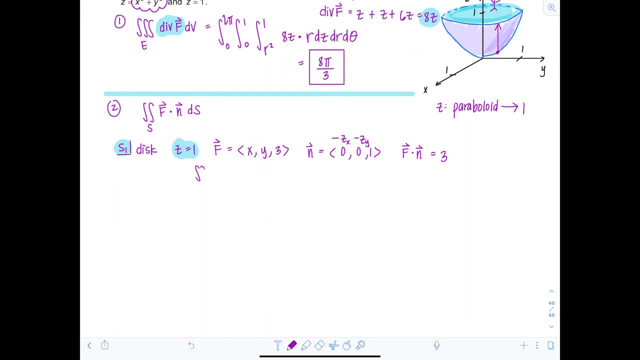 All right, very good. So from here let's find the flex On that first surface on the disc. so f, dot n, d s. Now I'm going to evaluate it as a double integral over the region D, And the region D is just going to be unit circle in the xy plane. 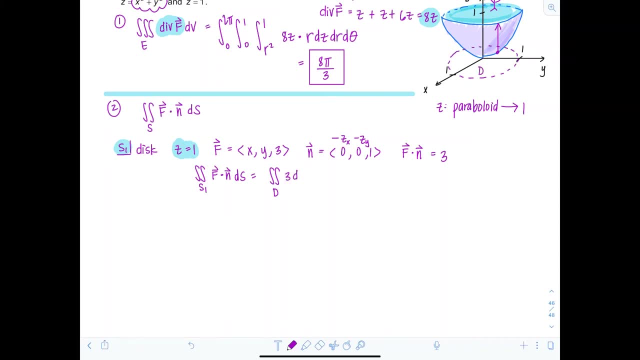 right, That's the easiest thing to do: 3 d, a, And I actually don't even need to set up an integral, because this is just three times the area of D, which is a unit circle. So pi r squared is just pi. So the flux on that surface is equal to three pi. 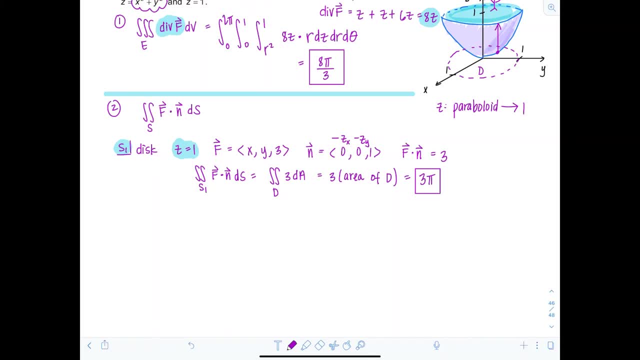 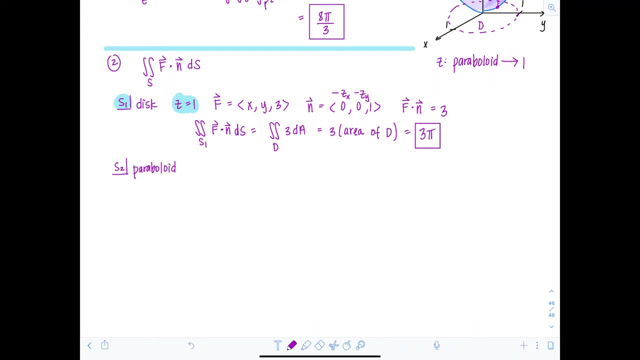 All right, now I'm going to move on to the next surface. So surface two is the paraboloid. Okay, so the paraboloid is determined by the equation z equals x squared plus y squared. Now I'm going to substitute that. 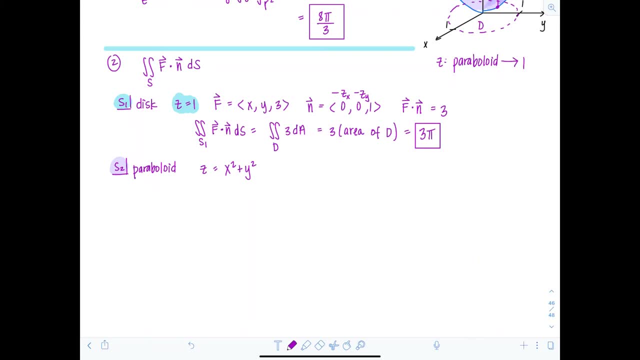 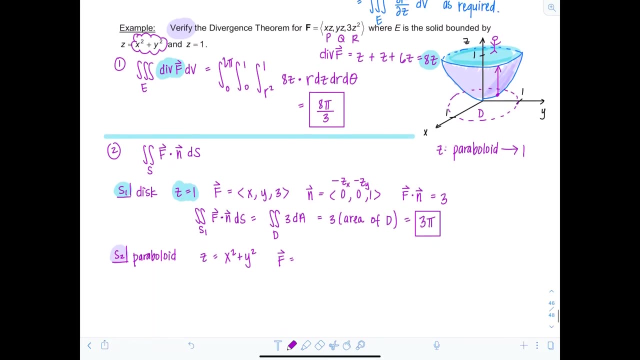 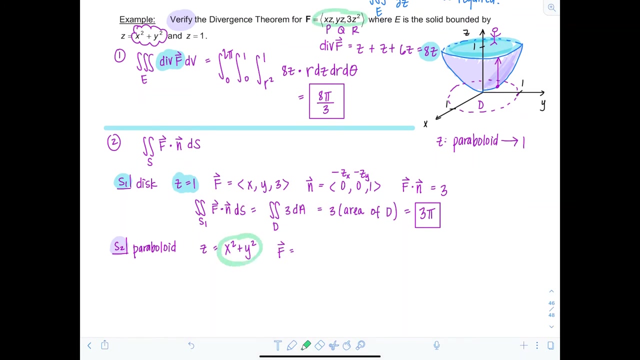 For z into my vector field. Remember: surface integrals are double integrals. You only want two variables going on, So f. if I need to remind you, it's up here. So xz, yz, three z squared. So I'm going to substitute this in everywhere I see z in the vector field. So I'm going to have x times. 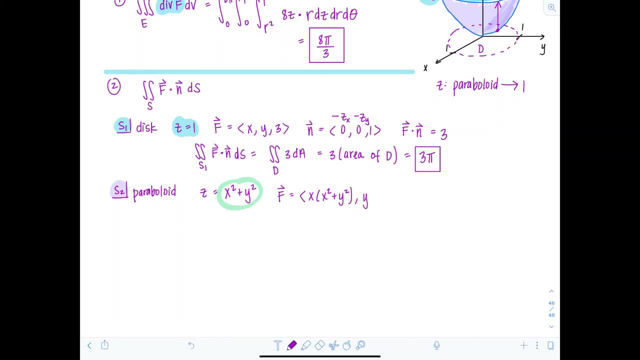 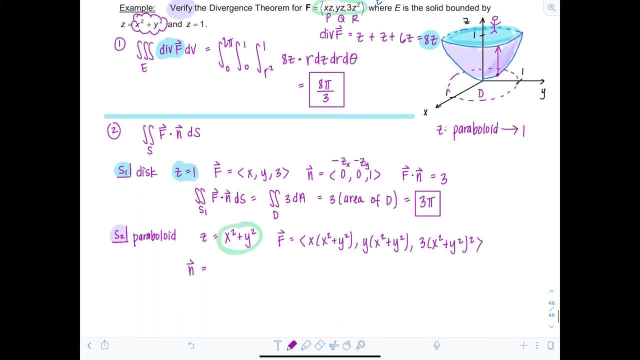 x squared plus y squared. y times x squared plus y squared. And then three times x squared Plus y squared squared. All right, what's the orientation of the normal vector? Well, you're walking on the paraboloid, The easiest way to figure out what the proper orientation. 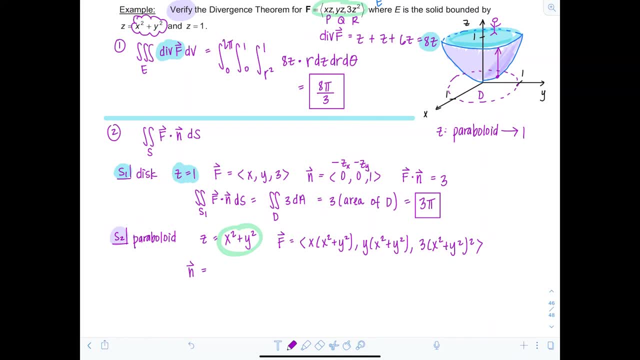 is is to imagine yourself at, like, the extreme points on the surface. So I would look, you know, at the vertex of the paraboloid And if I was walking on it my head would be pointing in the negative z direction. So that tells me that the z component is going to be negative z. So I'm going 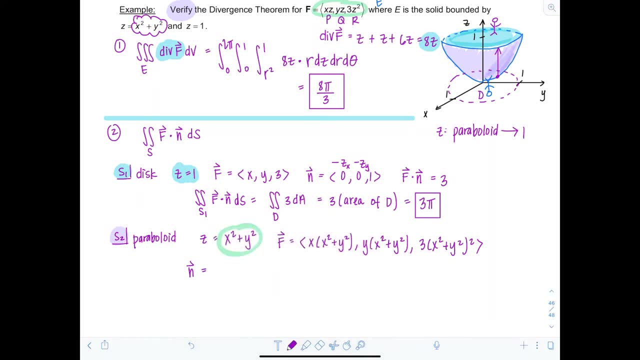 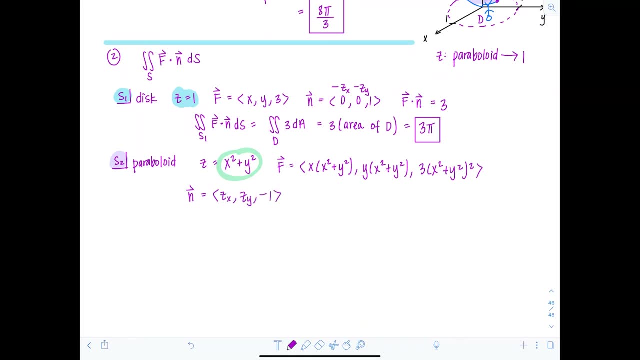 to have: partial with respect to x, partial with respect to y, negative 1.. Okay, you're taking partial derivatives of the paraboloid. That's the surface we're talking about. So I'm going to have 2x, 2y, negative 1.. And then let's go ahead. take the dot product f, dot it with n, Do all this. 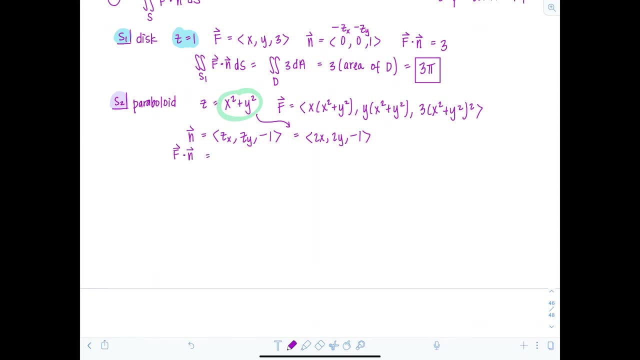 before you write out your integral: Okay, so you're going to take 2x times the first component, So that's going to be 2x squared times x squared plus y squared plus 2y squared plus x squared plus y squared minus 3 times x squared. 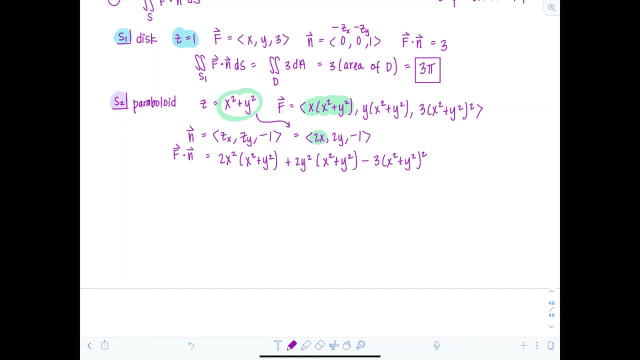 plus y squared, squared. And by all means don't you dare even try to multiply it out. No, no, no, Notice. they have a common factor. I can take an x squared plus y squared out of everybody, Yes, And then what are we left with? I'm left with. 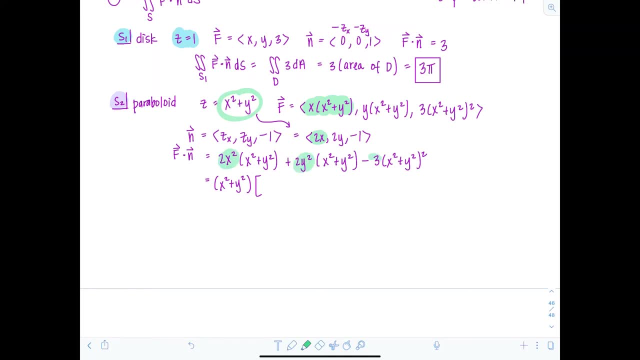 a 2x squared, a 2y squared and a negative 3 and just 1x squared plus y squared. Much better: 2x squared plus 2y squared, minus 3 times x squared plus y squared. All right, I can clean all this. 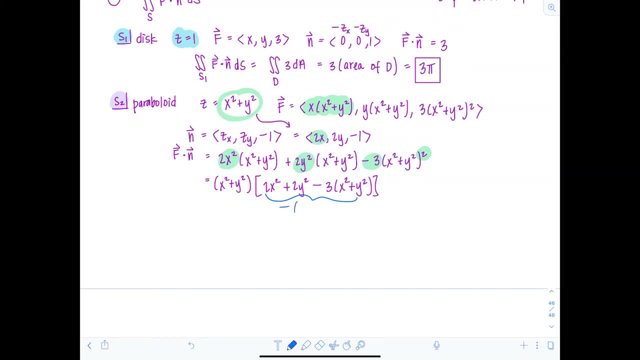 up easily. This is just negative x squared plus y squared, And lo and behold, f dot n cleans up really nicely. I just have negative x squared plus y squared squared. Voila Fabulous. So here we go. Let's find the flux on the paraboloid surface 2,. 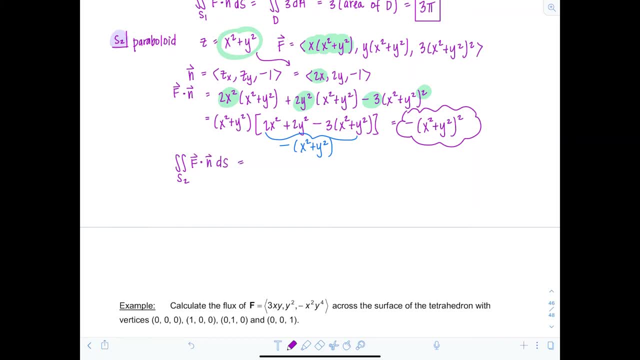 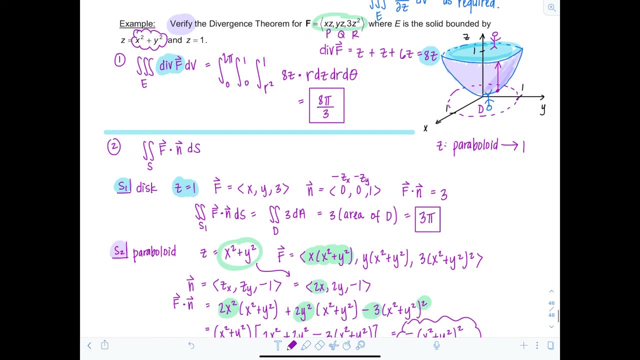 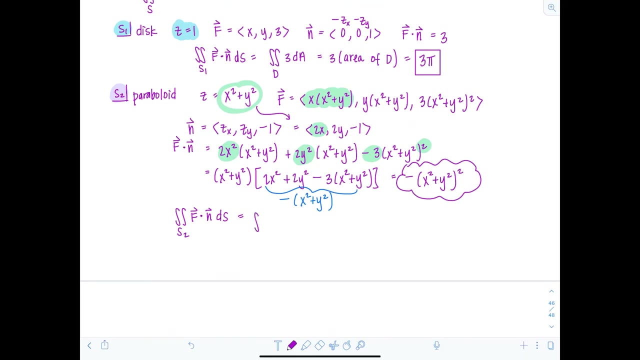 f, dot, m, d, s. So we're going to be integrating over d, which is in the x y plane. So look at the paraboloid. Same thing is just that unit circle. Let's switch to polar. Okay, I'll do that in a hot second, So double. 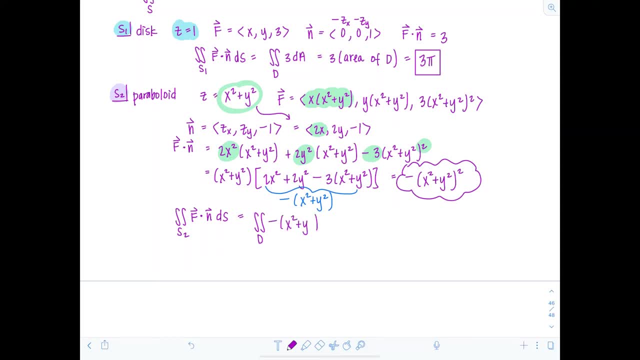 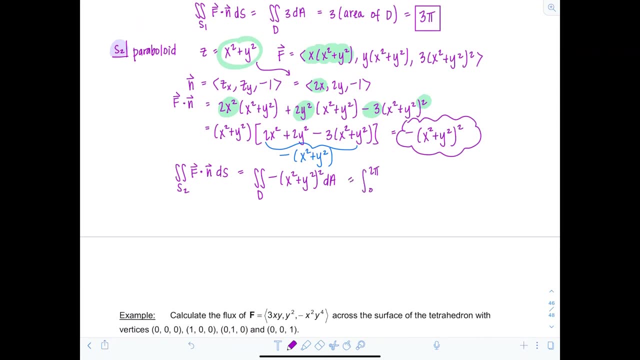 integral over d negative: x squared plus y squared squared dA. Okay, we're going polar. So this is going to be 0 to 2 pi for theta, 0 to 1 for r. Now, x squared plus y squared is r squared. So I have 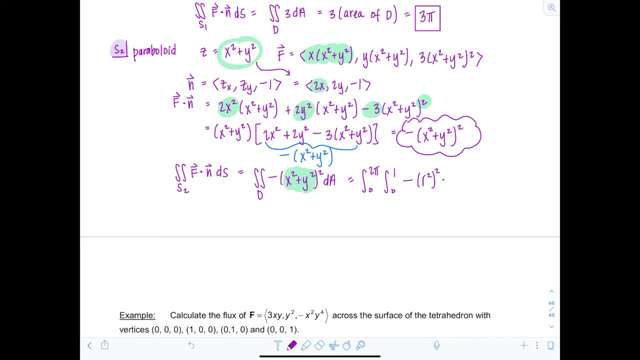 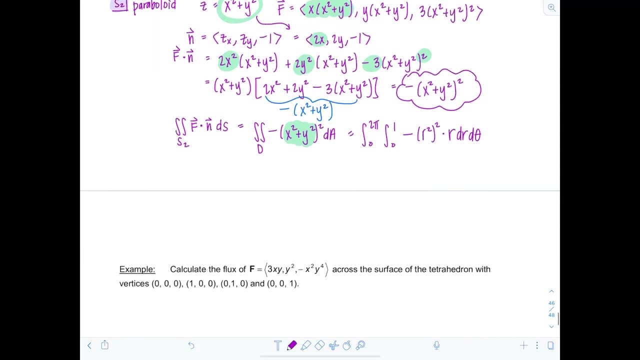 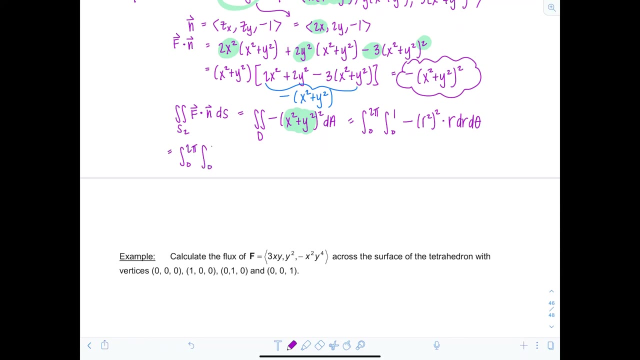 negative r, squared, squared. and then, don't forget extra r, dr d theta. Good. And then this is a nice, easy integral right, The worst part's over. So we have integral 0 to 2, pi 0 to 1, negative r to the fifth, dr d theta, which is negative pi over 3.. Now wait a minute. 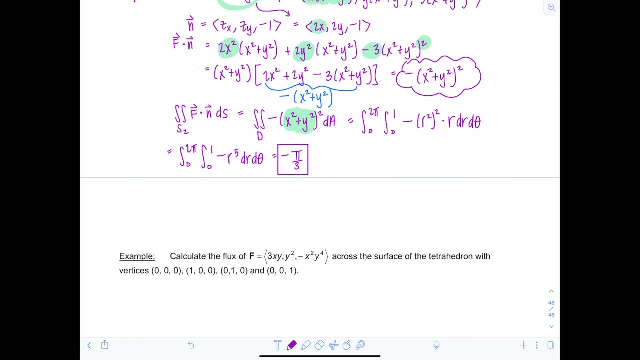 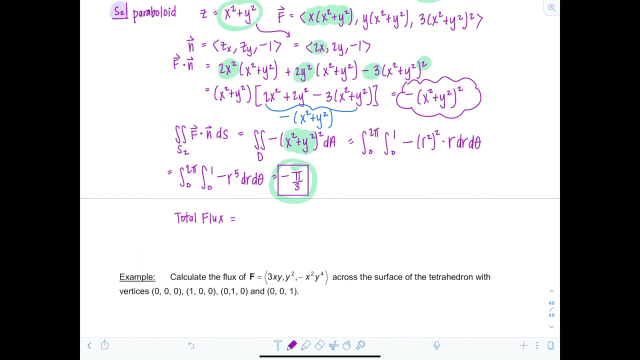 What do I have to do with this? I have to add it to the flux that I got on the disk to get the total flux. So the total flux for the solid is going to be 3 pi plus negative pi thirds And, my goodness, that's 8 pi over 3, which is what we got when we used the divergence. 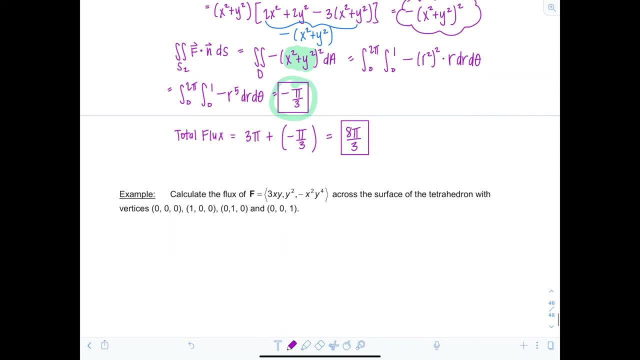 theorem and evaluated the triple integral over e. So both methods I can do like this, where I put in theаш and R, x, squared the same value, give the same value, or they gave the same value whatever. So the theorem is verified. 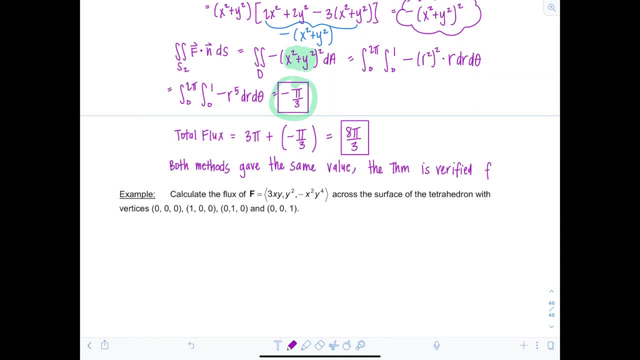 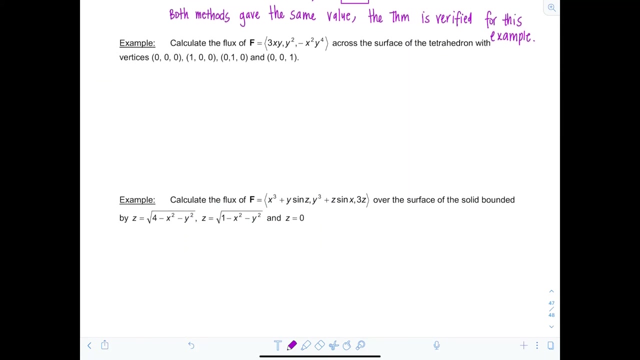 for this example. Okay, we did what they wanted, Very nice. Now let's look at a few more applications. applications, And don't worry, we won't have to do all of them as a surface integral and as a triple integral. That was just for fun. Here we go. Calculate the flux of the following vector: 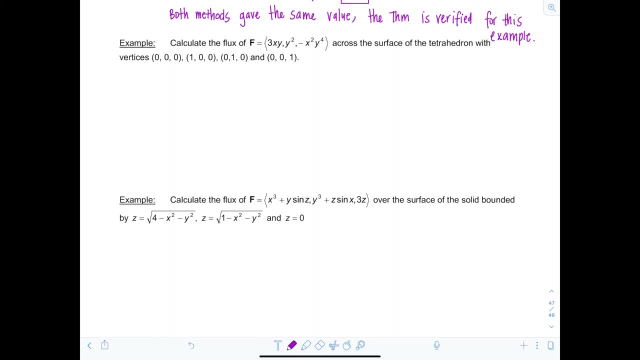 field across the surface of the tetrahedron with vertices 000,, 100,, 010, and 001.. Do you know this tetrahedron? You've probably become good friends over the past few weeks. Okay, z, x, y, 1,, 1, 1.. 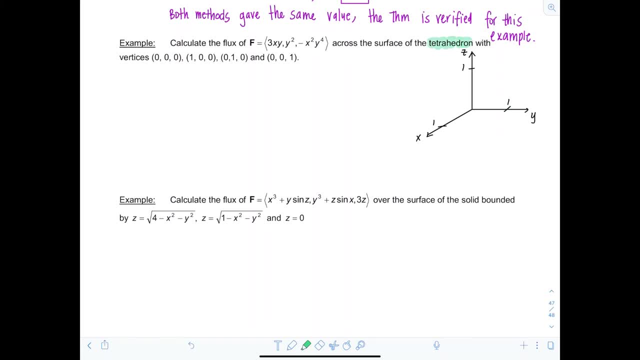 And notice, here it's a tetrahedron, So it's giving me the vertices, but this is a solid, This is a solid. So how many surface integrals would we have to do? 1,, 2,, 3, 4.. Four surface integrals, Or we could just apply the divergence theorem. 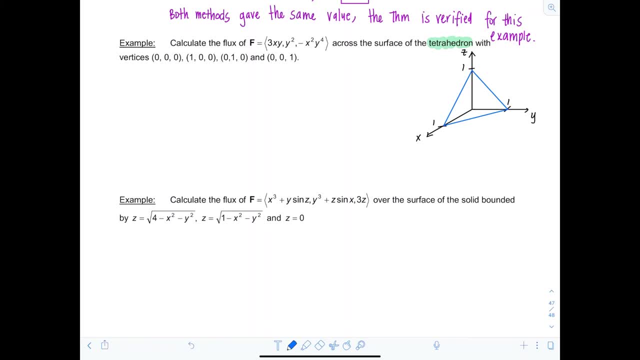 and do one triple integral. All right, we have a solid. Let's figure out what the divergence is going to be for the vector field and then determine how we want to integrate over the solid. I think the easiest thing is just to use the xy plane as 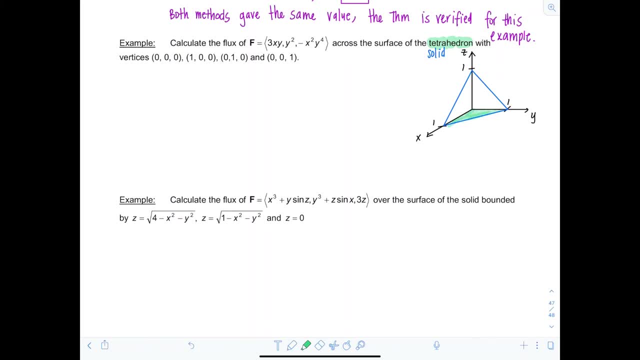 the base of the solid, And then we're going to use the xy plane as the base of the solid, And then we're going to use the xy plane as the base of the solid, And then we're going to use the equation of this plane here And we can use that as the height. Well, we know what that's going to. 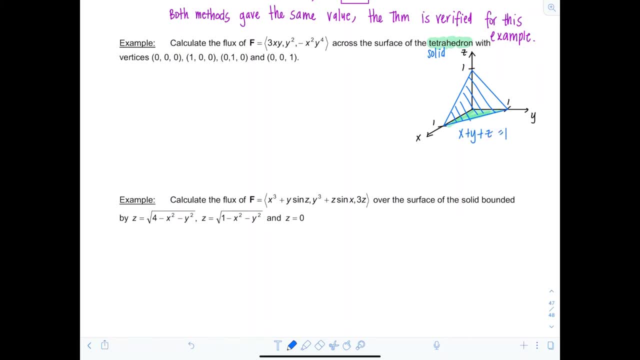 be That's x plus y plus z equals 1.. So I could just solve for z, z equals 1 minus x minus y, Easy stuff. Okay, let's get the divergence of our vector field. So partial derivative of 3xy. 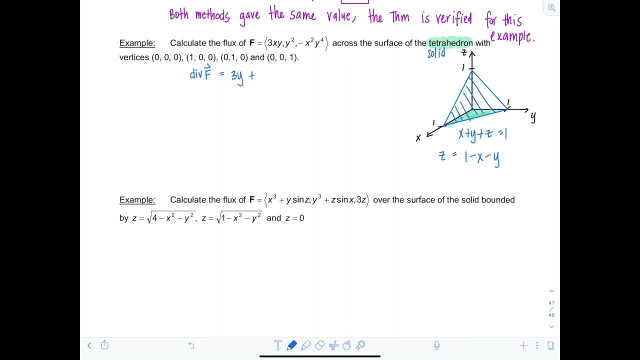 with respect to x is going to be 3y, plus partial of y squared with respect to y is 2y, And there's no z in the last column. So we're going to use the divergence theorem And then we're going to. 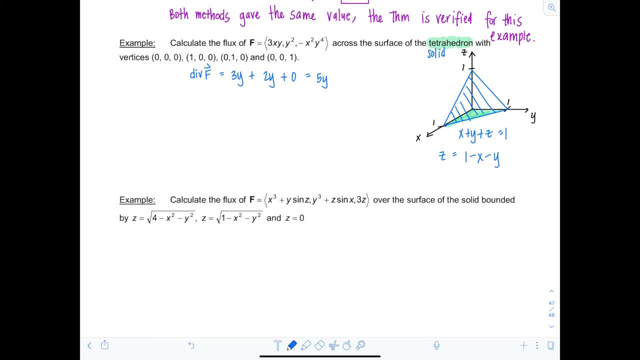 component. So this is just 5y. Okay, good, This is nice. Now, if I'm going to use the xy plane as my base region, let's see how we're going to set up this triple integral. Okay, so here's y-axis. 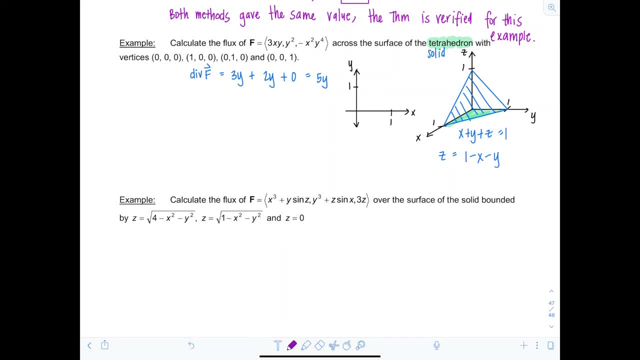 x-axis intercepts are both: 1. Make sure you shade in the appropriate region. I'll use the same color. And this is just: x plus y equals 1. So you can just as easily solve for x or y, But typically we solve y in terms of x. So our triple integral over e of divergence of f was: 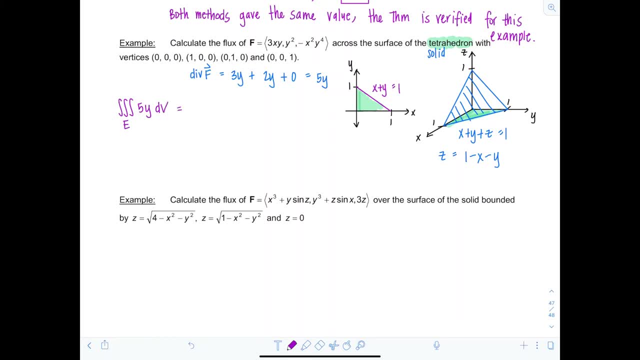 5y dv. This equals, I'll put limits for x on the outside. Okay, constant limits on the outside, 0 to 1. Limits for y would be 0 to 1 minus x. And then limits for z. notice z starts at 0,. 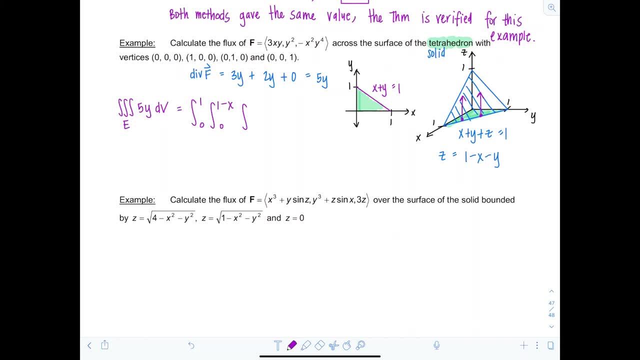 stops at the plane, Starts at 0,. stops at the plane, So starts at 0,. plane 1 minus x, minus y, and then I have 5y, dz, dy, dx. This is flux. If you want to write that every time to remind yourself, it's a good idea. And you get 5 over 24.. Okay, good. 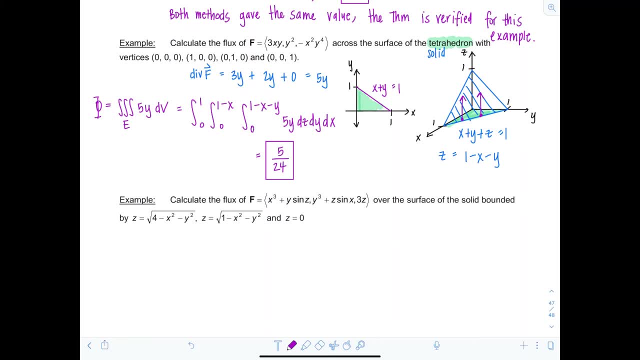 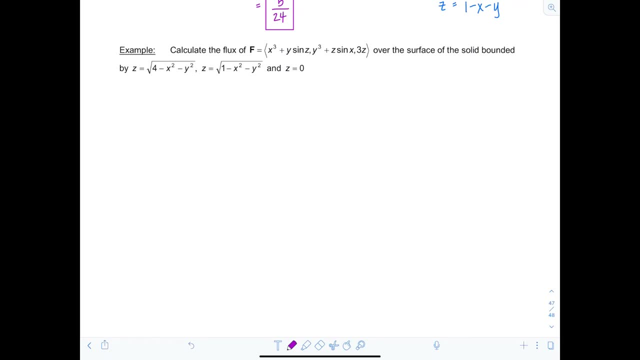 Let's look at another example where we're going to use a different coordinate system. Okay, so calculate the flux of the following vector field over the surface of the solid bounded by: z equals rad 4 minus x squared, minus y squared, and z equals rad 1 minus x squared. 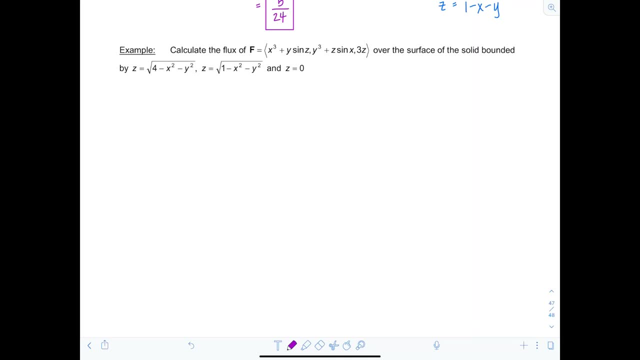 minus y squared and z equals 0.. So let's see, We're above the xy plane, and then these are two hemispheres, So our solid is bounded by these two hemispheres and the xy plane. Interesting looking thing. Okay, let's sketch it out. 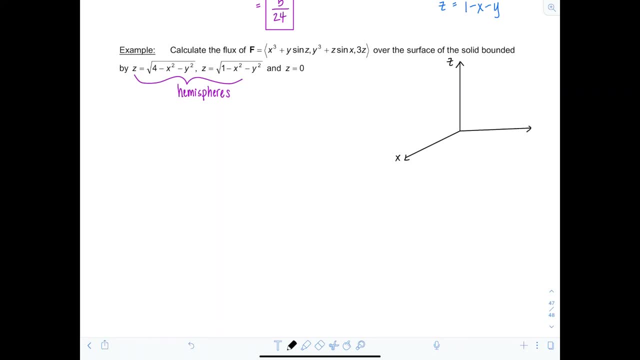 I mean, do you have a feeling for what coordinates this one? we're probably going to use Radius on one of the hemispheres is 2. We're working with spheres. if that's a hint, Okay, it's just the upper half, right, Because we only have the positive radical. 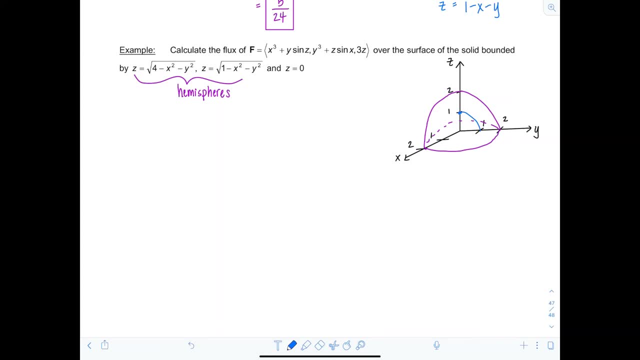 And then we have another one. Radius is only 1. And the solid is bounded between these two And the plane z equals 0. Okay, so it lies in between these two and it's bounded below. All right, let's go ahead. first, find the divergence of our vector field, So divergence of f. 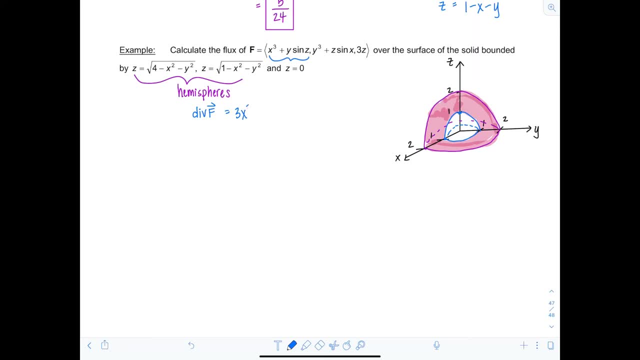 So partial of the first component with respect to x is just 3x squared Plus. this is going to be 3y squared plus 3.. Okay, now I'm looking at this solid E and it seems like spherical is going to be the way to go. 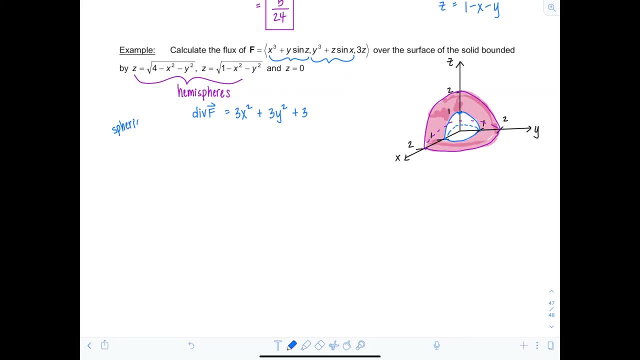 If I'm going to integrate over this solid spherical, So let's switch 3x squared plus 3y squared plus 3 into spherical coordinates. So easiest thing is take the 3 out, So you have x squared plus y squared plus 1.. 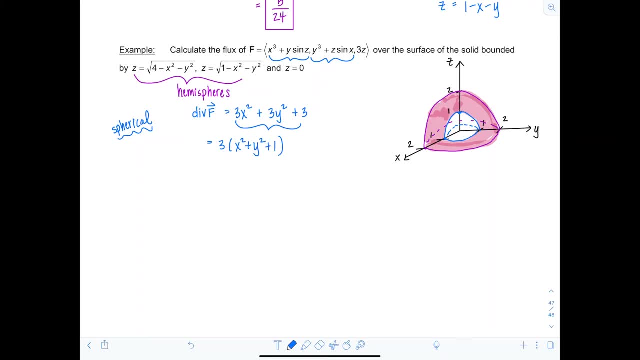 And then you can make Like a little pit stop in cylindrical land before you go all the way to spherical coordinates, if it helps. So this is 3 times r squared plus 1, right, And then you go: oh, that's right, r is rho sine phi. So this is 3 times rho squared sine squared phi, plus 1.. 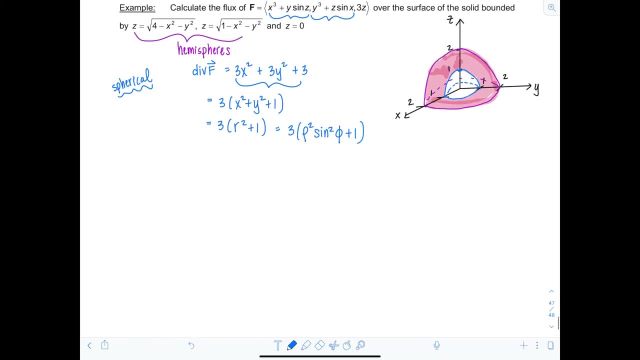 Awesome. So that's what we're going to be integrating. So flux is going to equal. Let's take the 3 outside Now limits for theta We need all the way around. So theta is going to go from 0 to 2pi. 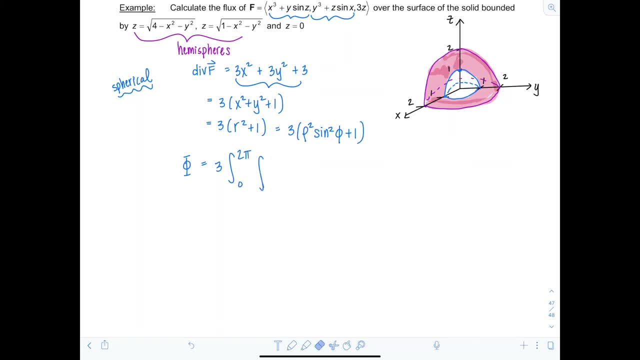 What about limits for phi? Well notice, here we only need the upper half. So phi is going to go from 0 and stop right there at the positive y-axis. So phi is just going to go from 0 to pi-halves. 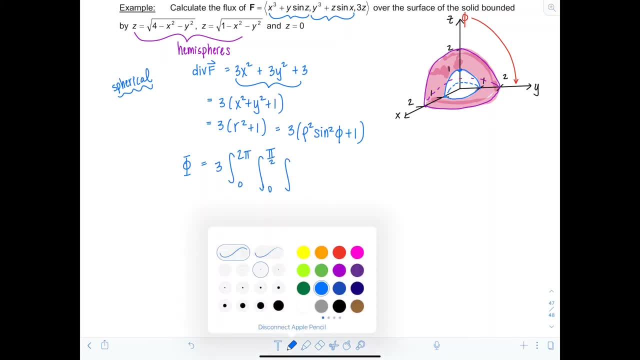 And then what about rho? Well, rho needs to start at the inner sphere hemisphere, and go to the outer one. So rho is bounded below by 1 and above by 2.. So the limits for rho are going to be 1 to 2.. 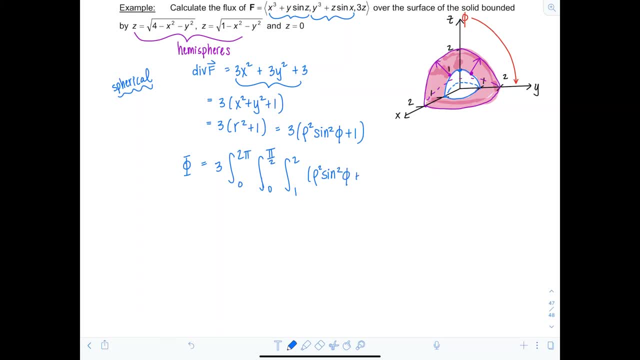 And then I have rho squared sine squared phi plus 1.. That's what's left of the divergence of F. Remember I already took that 3 outside? And then dv? do you remember what it is in spherical? Yes, it's rho squared sine phi. 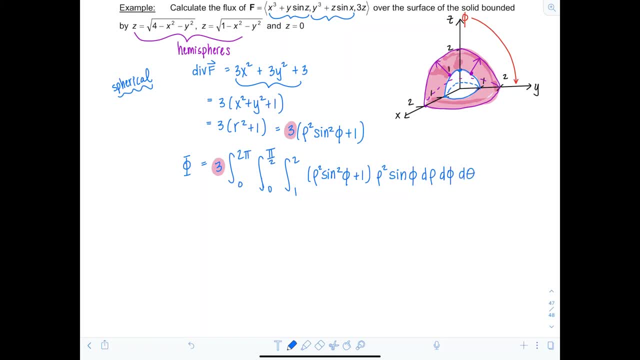 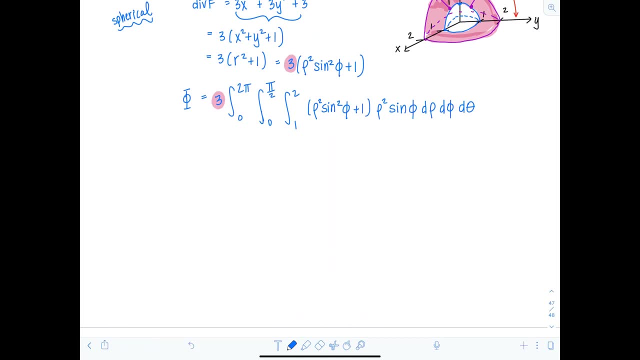 d rho d phi d theta. Okay, I'm not going to sit here and evaluate the whole thing with you, but we'll just do some tips. I don't see a single theta in this thing. right, So, right away, you're going to multiply the whole integral by 2pi. 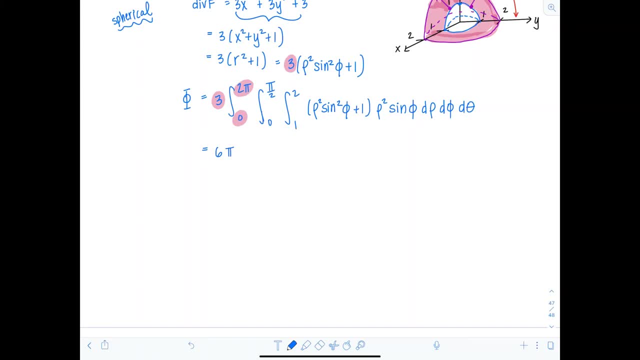 which means I'm going to have a 6pi sitting outside, And then you have 0 to pi-halves, 1 to 2, and then no shortcuts from here. This is rho to the fourth, sine cubed phi plus rho squared. 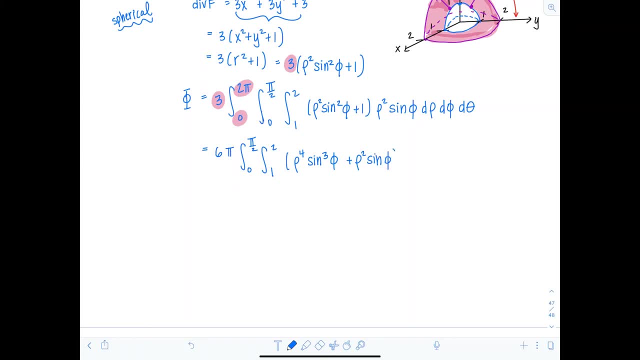 sine phi d rho d phi. Okay, and then just confirm that you can get 194 pi over 5.. Oh my, that's the answer. Okay, Last one, last example. I'm a little sad about it. Okay, so far, when we've been finding flux, remember it has to be a closed solid. 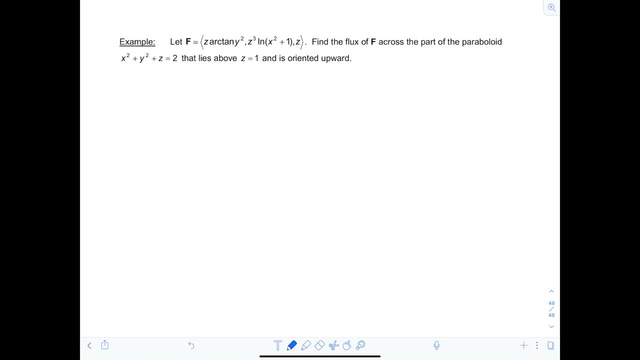 But what if you don't have a closed solid? We can work around it, don't you fret? So here's a vector field. Cool, Find the flux of f, that vector field, across just the part of the paraboloid. 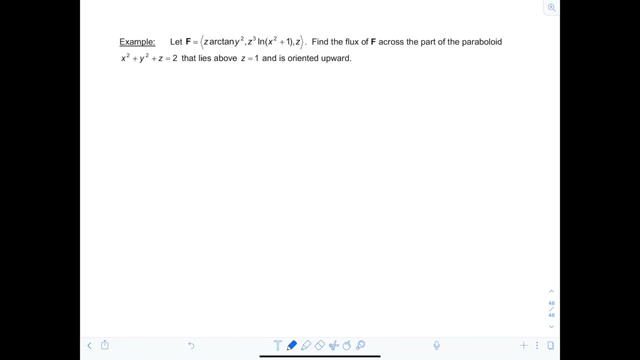 x squared plus y squared plus z, equals 2. that lies above z, equals 1, and is oriented upward. See, so they only want flux across the paraboloid. x squared plus y squared plus z, equals 2. that lies above z, equals 1, and is oriented upward. 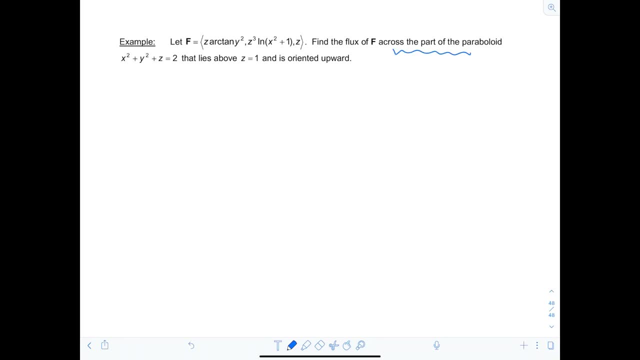 See, so they only want flux across the paraboloid x squared plus y squared plus z equals 1 and is oriented upward. See, so they only want flux across this part of the paraboloid: x squared plus y squared plus z equals 1 and is oriented upward. 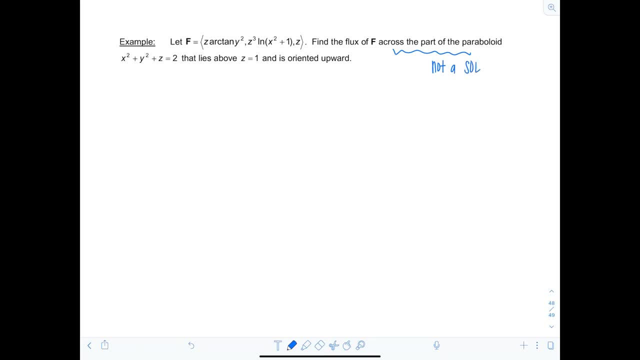 So that means it's not a solid, And when we find flux using divergence theorem, it gives us the flux over the entire solid. So it's not going to give us the right answer if we use the divergence theorem, unless we subtract the flux on the part of the surface that we don't want. 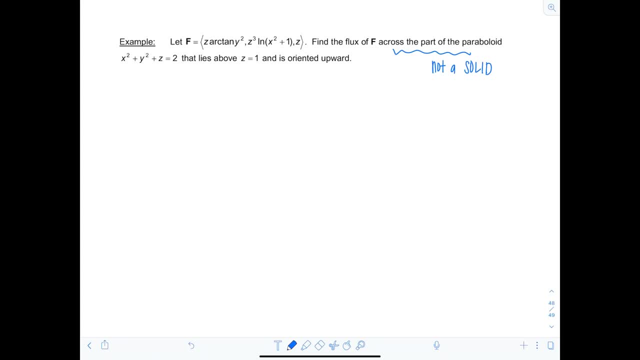 Okay, I'll show you exactly what I mean. Okay, I'll show you exactly what I mean. First of all, maybe this equation isn't looking like a paraboloid to you, So you gotta solve for z and you go. oh, now I see it's been shifted 2 units upward. 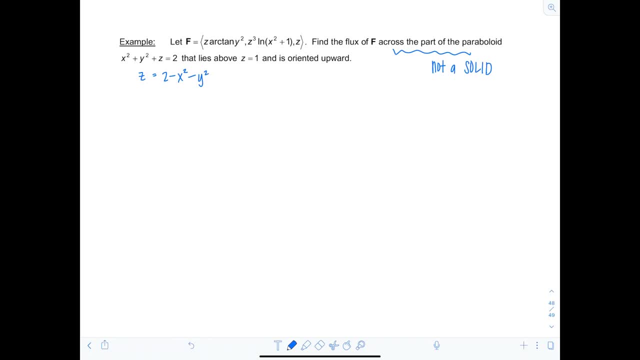 two units upward and it's opening downward. Okay, fantastic. What's the divergence of this vector field? It'll make you feel better instantly. Look at this. not a single x. Next component, not a single y And lastly, this is one. My goodness, aren't you glad we don't have to do? 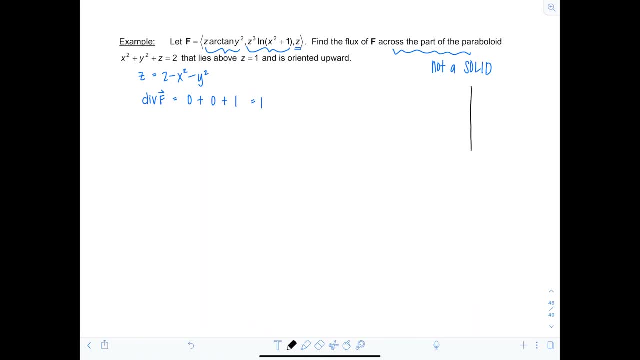 a surface and it would be a little nasty. So here we go, let's draw the paraboloid and see what's going on. Z, x, y, it's been shifted up, two units, Okay. and then I know it's going to intercept the. 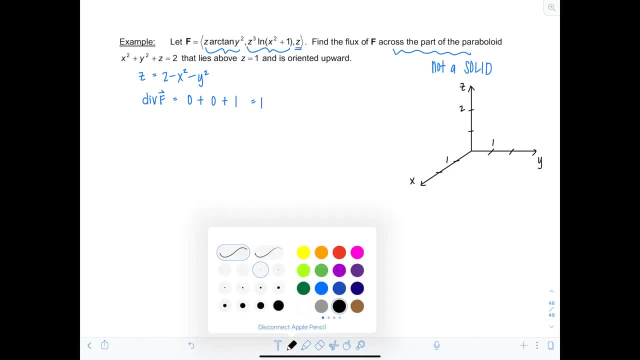 xy plane at a circle whose radius is going to be rad 2.. Yeah, so somewhere around here up here. But I only want the flux on the paraboloid that lies above z equals 1.. Okay, well, where does it intersect with z equals 1?? 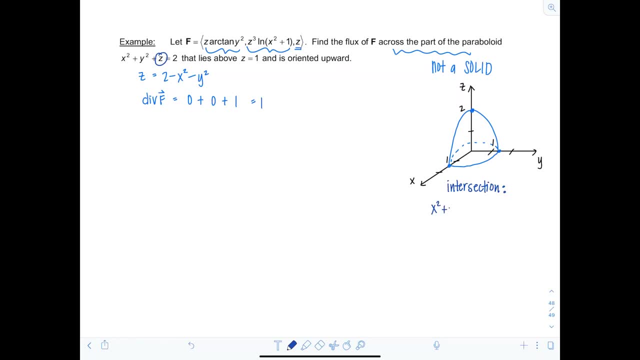 Well, I'll just substitute in 1 for z here. So I get x squared plus y squared plus 1 equals 2.. So it intersects in the unit circle at z equals 1.. So basically, right here, You see, it's a unit circle. 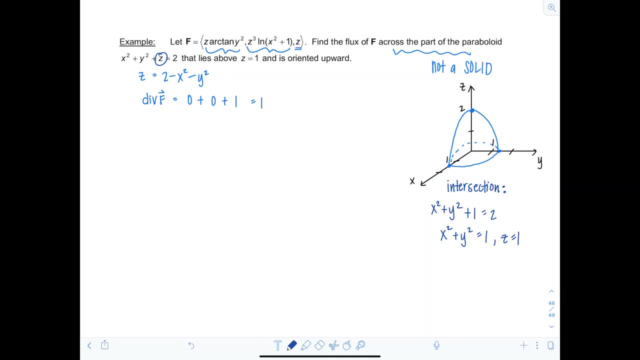 Okay, Let me draw a better one. I'm not pleased, Not at all. Oh, much better. Okay, there's the equals one. So I only want the flux for this portion of the paraboloid And I don't want to include. 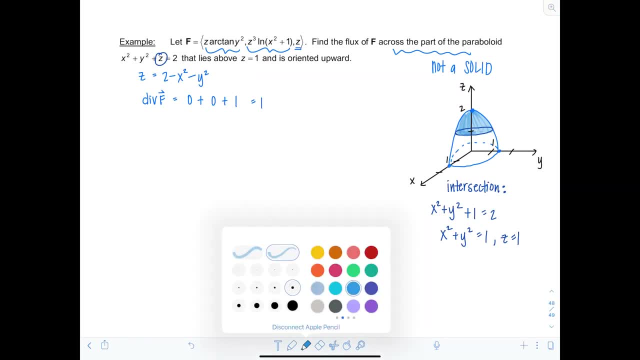 that base, The base being this circle right here. Okay, so how do we start? You don't worry. So you evaluate the triple integral over the solid E of the divergence of F- dv And remember that's going to give us the total flux. 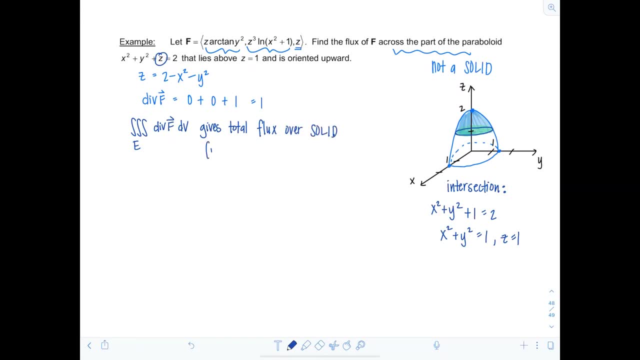 over the solid And then we need to later subtract the flux on the base. But that's going to be a much easier surface integral to evaluate than doing the surface integral. I mean, look at the spectrum. We're going to be doing the surface integral over the paraboloid. 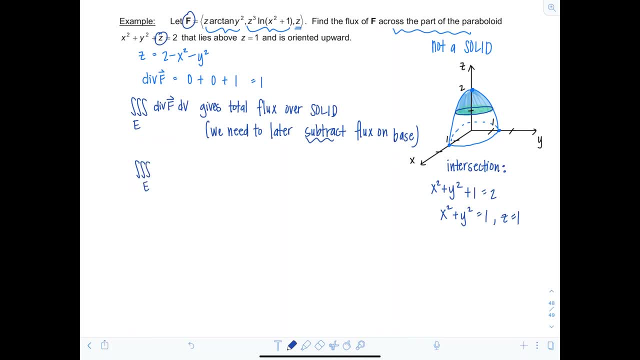 Okay, so triple integral over E. divergence of F was just one, We love it, dv. And then, if we're going to evaluate this triple integral, I need the volume of E. Let's use cylindrical right, It seems appropriate. So limits for theta should be 0 to 2, pi, Limits for r 0 to 1.. And then limits for z. Notice: z starts at z. 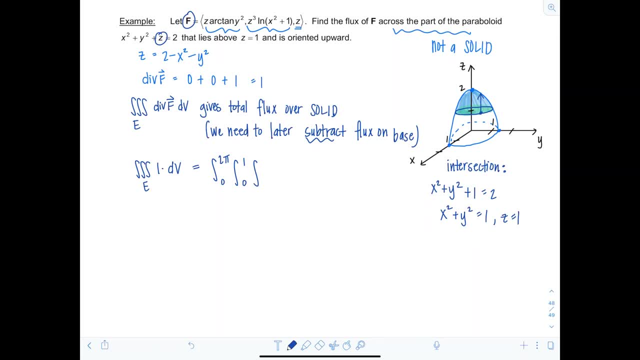 Starts at 1, ends at the paraboloid, So that would be 1, 2, 2 minus x squared minus y squared, so 2 minus r squared r dz. dr d theta, Okay, I'll let you play around with that. 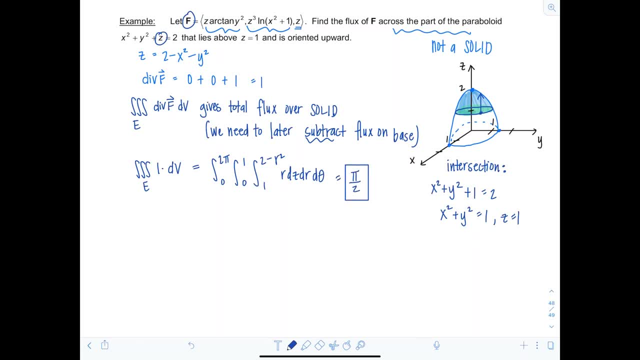 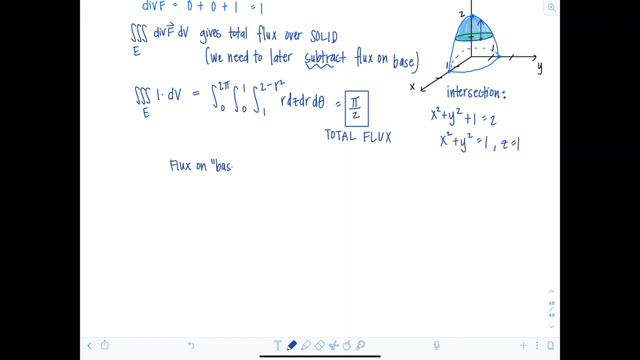 This gives us pi halves. So this pi halves represents total flux over the solid. Now, remember I need to subtract the flux on the base, The base being z equals 1, that little green circle I highlighted, Okay, good. So remember we need a surface integral for flux: f, dot, n, ds. 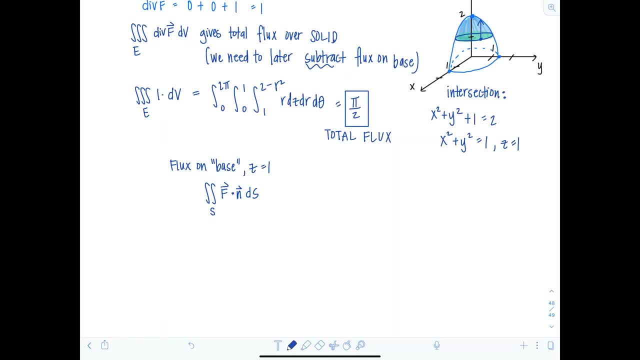 And I'm going to substitute 1 for z into the vector field. So I'm going to have 1 times 1.. 1 times tan inverse of y squared, So just tan inverse of y squared. And then 1 cubed times natural log of x squared plus 1.. 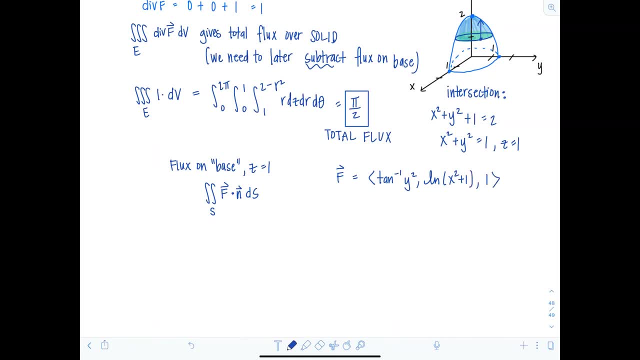 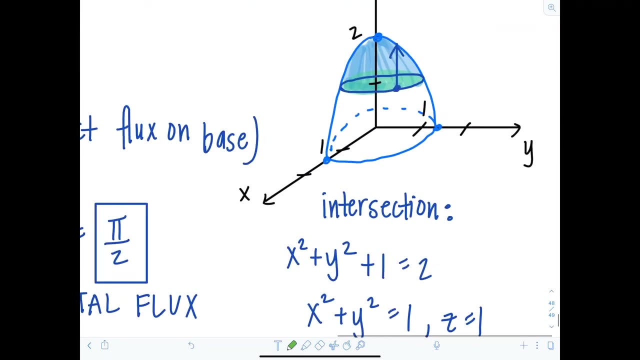 And then last component is just z, so 1. Now what's the normal vector? Imagine you're standing on the base Here, you are Decided to take a walk on the paraboloid And you made it to the base. 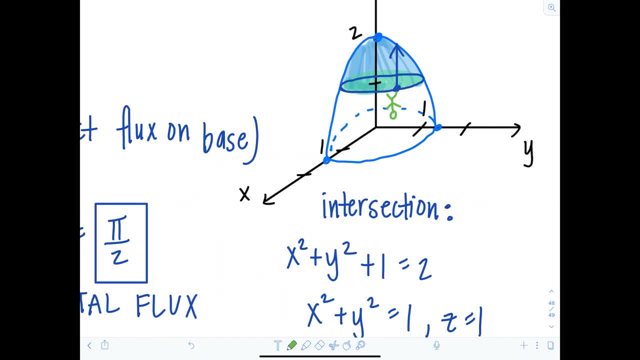 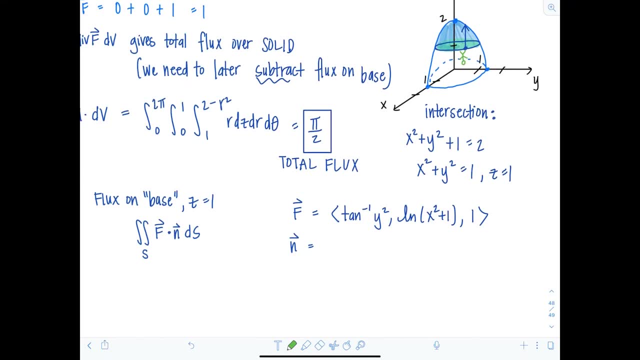 Which way is your head pointing In the negative z direction? Right, And it's just a plane. So the components are going to be 0, 0, negative 1.. Okay, So 0, 0, negative 1.. 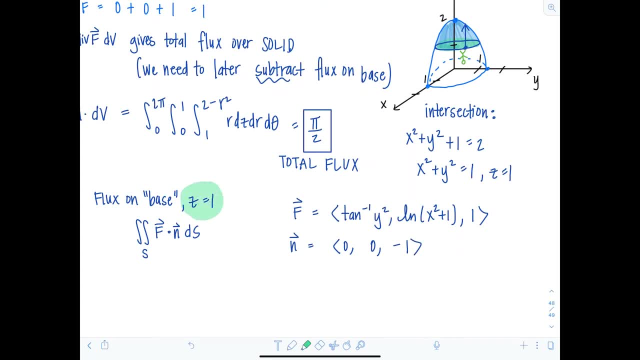 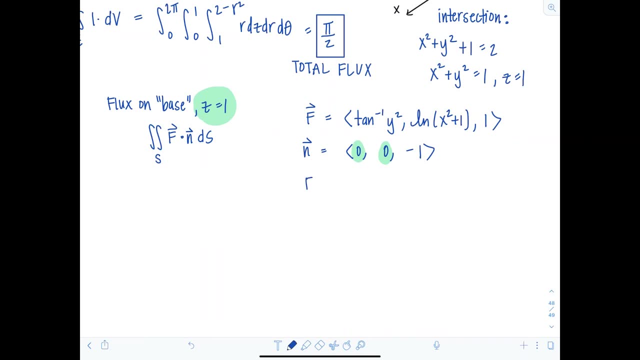 You could also take partial derivatives of this constant with respect to x and y. You'll get 0,, 0, and then negative 1.. Good, Well, look, that's our saving grace. f dot n turns out to be super manageable. 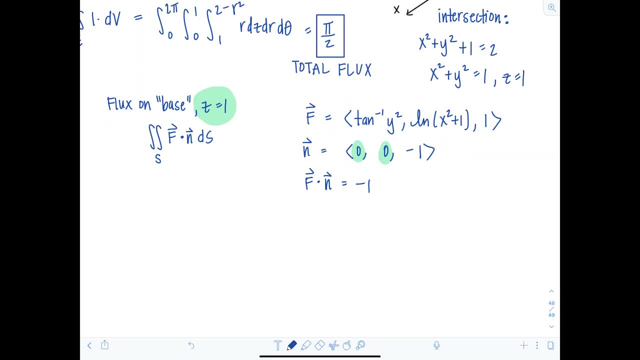 It's just negative 1.. So I think you guys can handle it. So we're going to handle. now, integrating this surface integral, It's going to become double integral over d of negative 1, dA. What's d? d is just the unit circle, right. 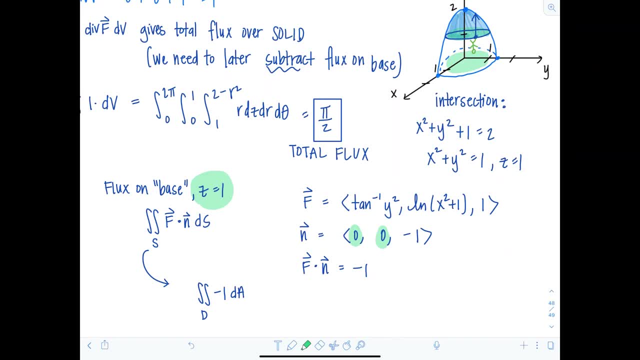 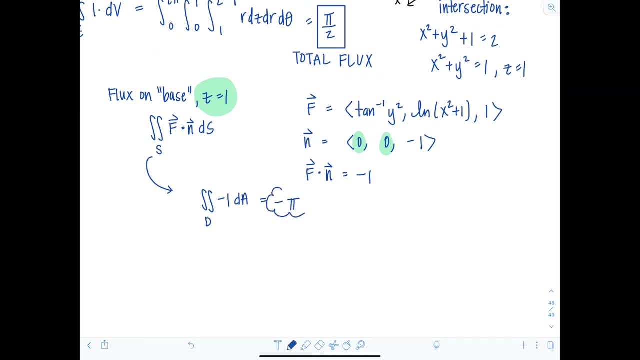 In the xy plane. That surface projected over the xy plane is the unit circle. So area is going to be pi times negative 1. So this is negative pi. Okay, So now we can just put it all together. That means the flux on the paraboloid. 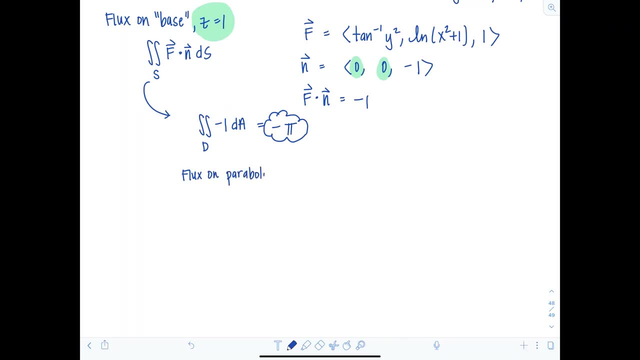 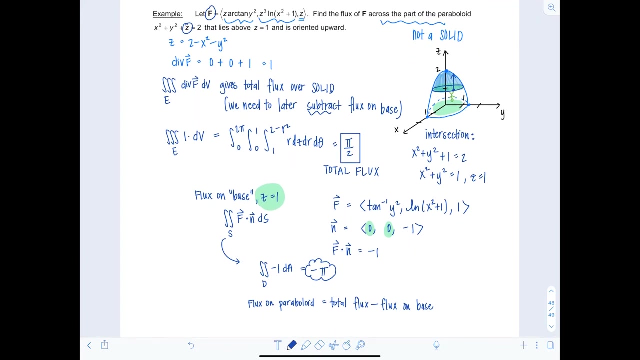 is equal to the total flux minus the flux on the base. And then let's see- here I'll zoom out so you can see it all together. Total flux was pi halves. Flux on the base is negative pi, So we have pi halves. 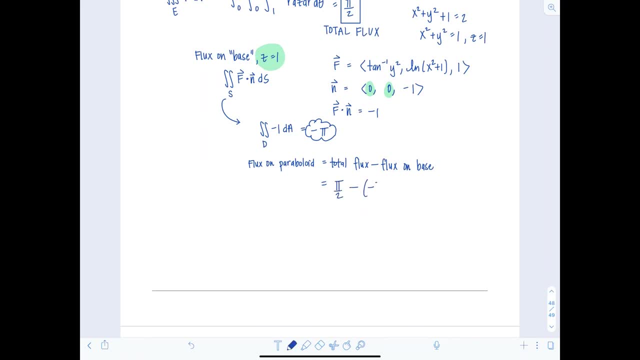 Minus negative pi, Which gives me 3 pi over 2.. So 3 pi over 2.. That is the flux on the paraboloid only Okay. So that concludes the lesson on the divergence theorem, As well as all of the videos on calculus 3.. 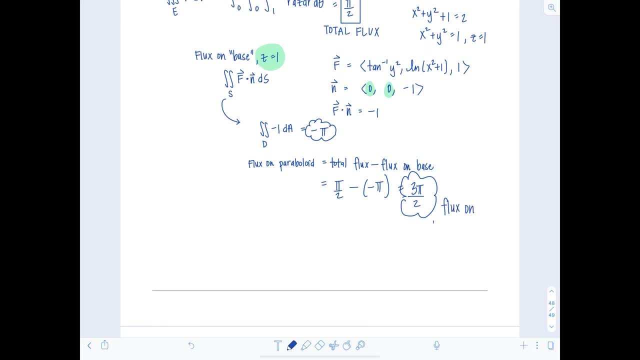 I hope you enjoyed it And if you have any questions, please let me know in the comments below. And if you have any questions, please let me know in the comments below. And if you have any questions, please let me know in the comments below. 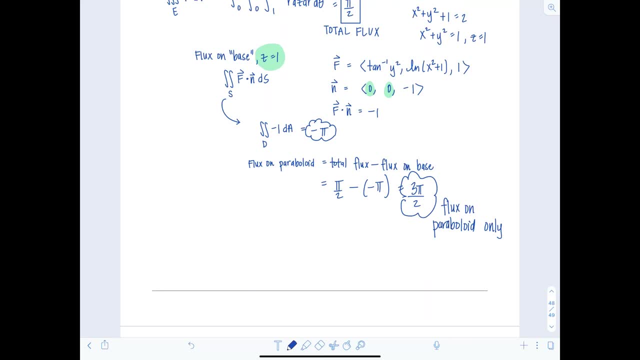 I hope you enjoyed it. It really is such a beautiful conclusion. It really is such a beautiful conclusion to your calculus journey. Don't forget to give this video a thumbs up. Comment down below what your favorite thing was that you learned. I hope you stay tuned for more videos.